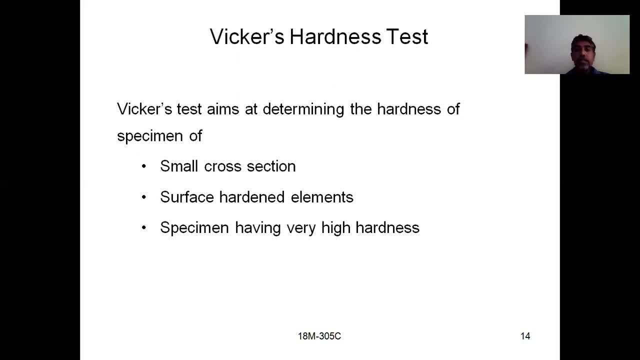 Because there we are using steel ball indenter. So by using steel ball indenter we are unable to find hardness of hard materials. So if you want to find out hardness of hard materials you have to go for Vickers hardness test. So why it is useful for hardness? 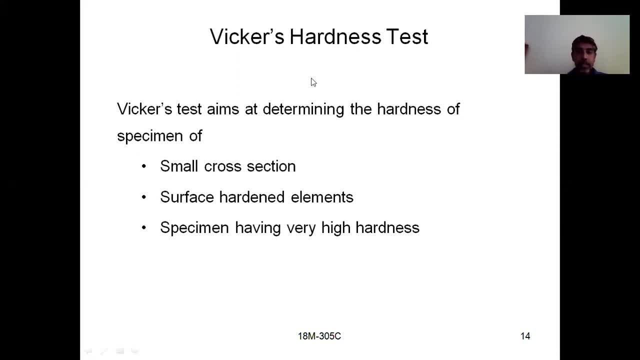 Because if you see these points here, if you see the points why we can use this one for harder materials, It can be useful for smaller cross section and it can be useful for surface hardened elements and is also useful for very high hardness materials. 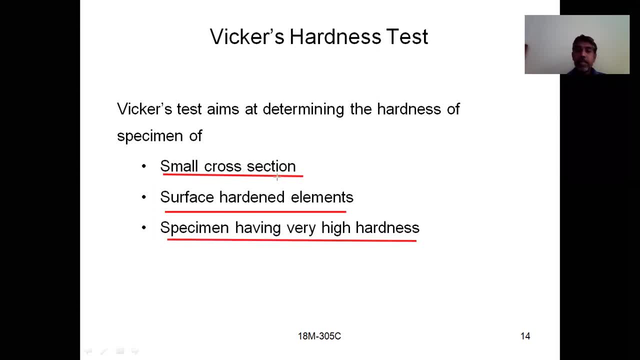 So why we can apply for small cross section materials and surface hardened materials. That means the core may be soft But the surface may be hard material. so for such material also we can use this Vickers hardness test, And specimen having very high hardness and materials having high hardness also can be tested by using this Vickers hardness test. 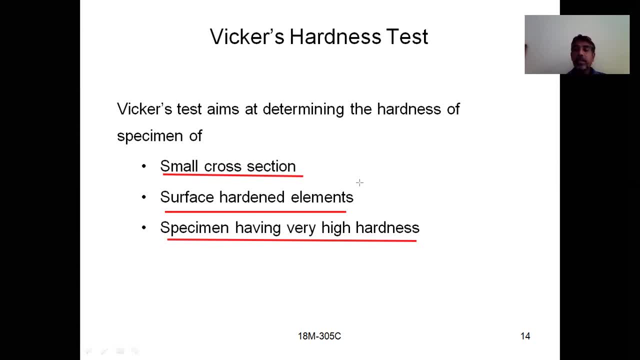 So why we can do all these things by using this Vickers hardness test? because here we are using a diamond indenter. Ok, So here we are using a diamond indenter. We all know that diamond is a hardest material compared to all materials, so such that we can use this diamond indenter. 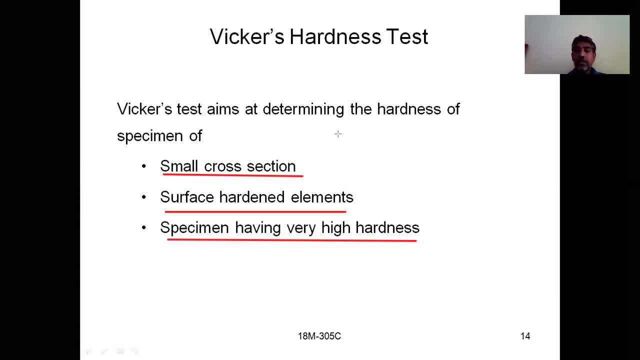 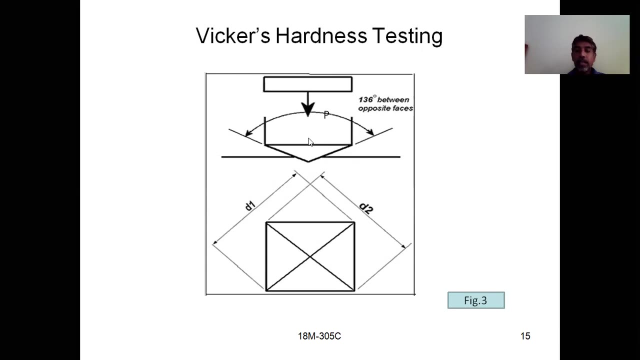 to test the hardness of very hard materials. also, If you see the next points, how the diamond indenter will look like, If you see here so how the diamond indenter will look like and what is the shape of that indenter, we will discuss in this slide. 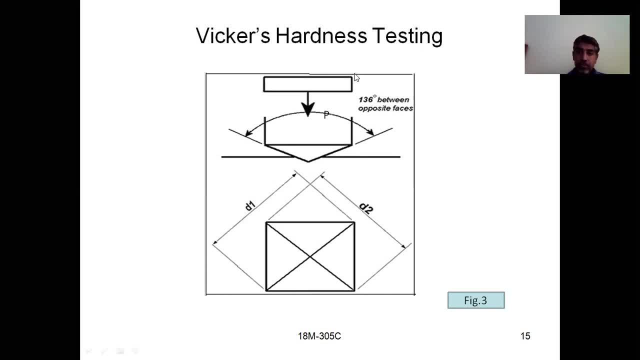 If you see here, if you see the diagram I will show, you See here, if you see this one, see this is the shape of the diamond indenter. and if you see this angle, how much angle you are having this one. 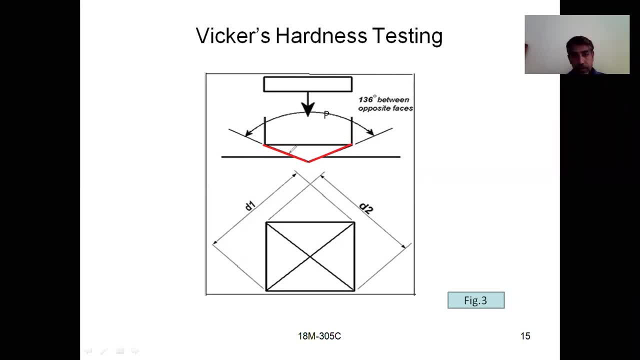 I will show the angle also. If you see the diagram, this one from here to here, how much angle it is 136 degrees. 136 degrees between the opposite faces. so here you are having a sharp corner, so you are having a sharp pointed edge here. so that's why we can use this one for small. 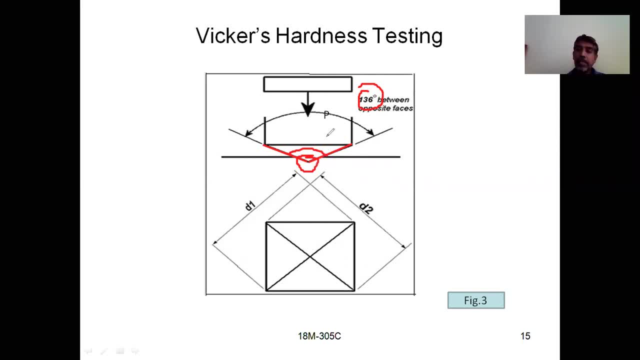 cross sections also and we are using a diamond indenter, so diamond in the diamond is very hard material, so we can use this one for testing of hardness of hard materials. so in this way this is is having some advantage compared to your Brinell hardness test. 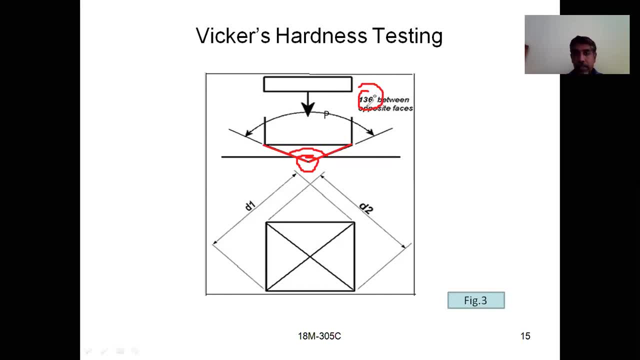 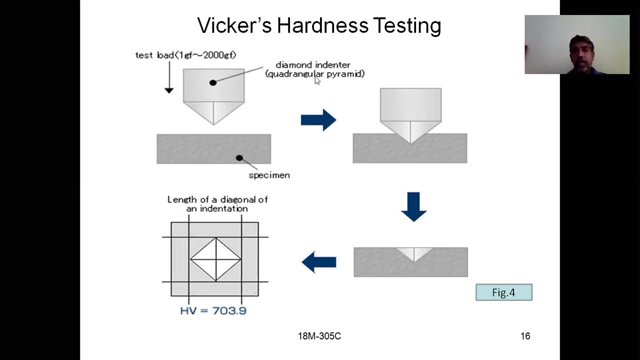 so how much angle between the faces, opposite faces? it is 136. so you should remember this value: 136 degrees between the opposite faces when you use the diamond indenter. so what is the shape of that in enter I will show you see this one. so if you see, here it is a quadrangular. 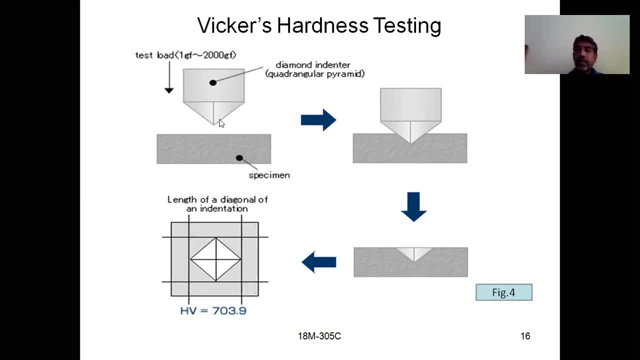 pyramid. so you are having four faces and you are having those four faces are joined with a sharp point here. if you see here this is a quadrangular pyramid. if you see here, so you are having four of these four interfaces. see so here, in this view, you are at visible only two. if 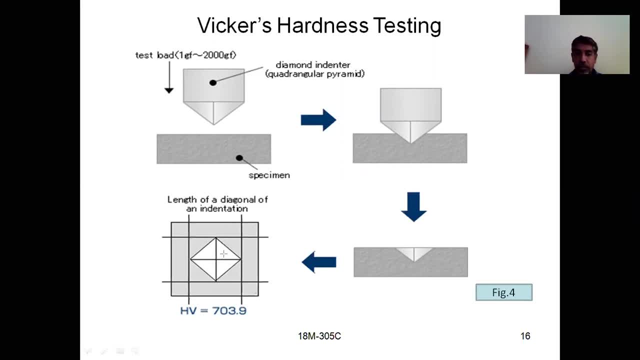 you see here, one, two, three, four. so one, two, three, four, these four phases are won too good. so phase front face: phase 2, phase 3, phase 4, 4 faces are joined here. See, here, at this point those faces are joined. So this is the top you are seeing, this is the front you are seeing, And it is. 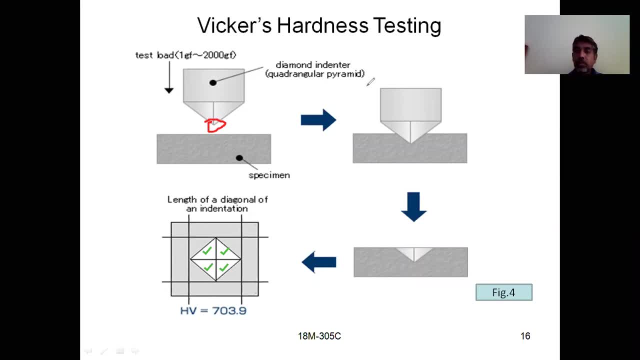 the quadrangular pyramid. So 4 faces are there and the shape is pyramid shape. So those faces are joined at a single point. So because of single point joining we can use for small cross section or area materials. If you see, here this is the area of cross section here. 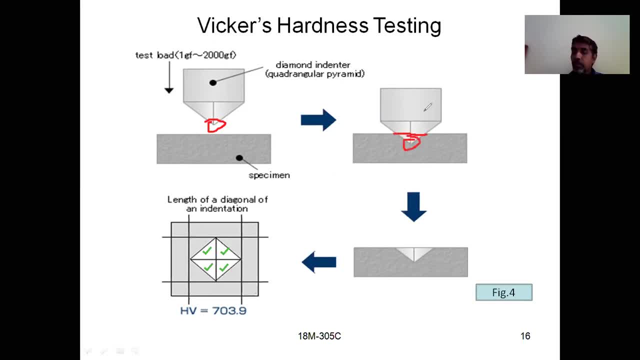 and you can have this much area of cross section also. So that's why we can use this indenter for very small cross section also. We are using this indenter because of that advantage. we can use Wickers hardness test for smaller cross sectional area materials. So what we 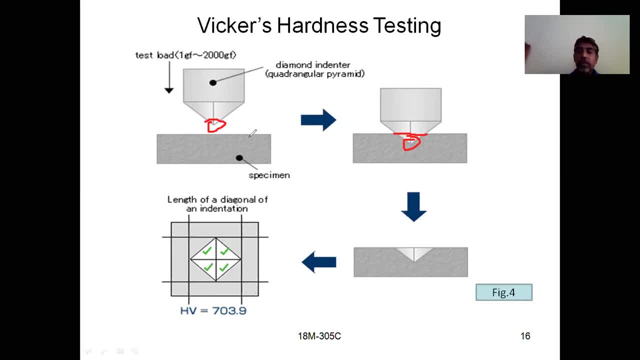 i have to do? What is the procedure? As usual, we have discussed in the Brennel hardness test that what you have to do, period, same thing. so first, what you have to do: you have to prepare the specimen and you have to keep the specimen under anvil and later you have to apply them. you have to move the specimen such that it 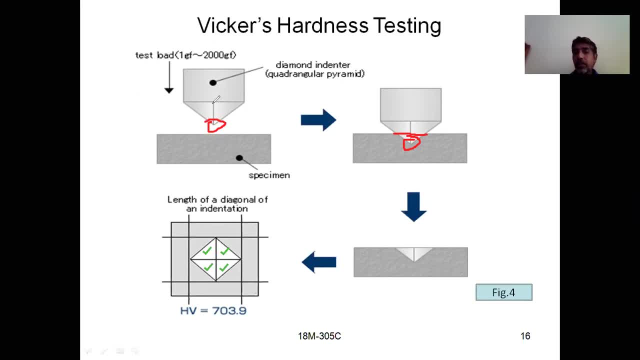 should touch the indenter and later you have to apply the load. when you apply the load, what will happen? if you see here- i will show you it clearly- if you see here what is happening- this indenter penetrate into the material, so so this much penetration will occur here. this much penetration. 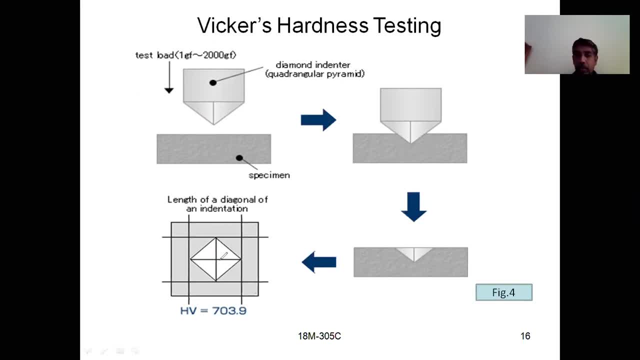 occurred here. so because of if you see the top, you you will get this view. so from the top you will get like this, and if you from the front, if you, if you see, you will, you will see like this. so when you apply the force, what is happening? the pen indent is penetrating into the material. 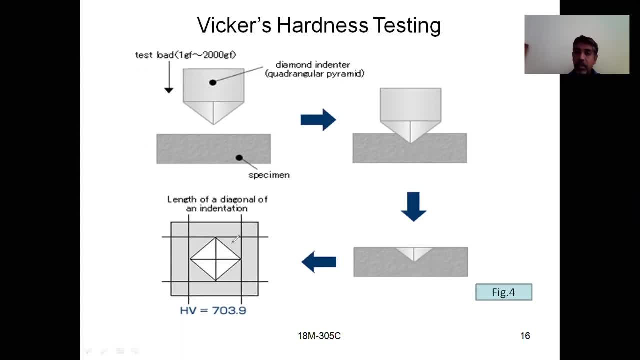 because of that one, you are getting indentation. so this is the shape of the indentation from the top view and this is the shape of the indentation from the front view. okay, and based on that indentation, we will measure the pyramid hardness number. okay, so how to find out the pyramid hardness number, i will show you. if you see here. 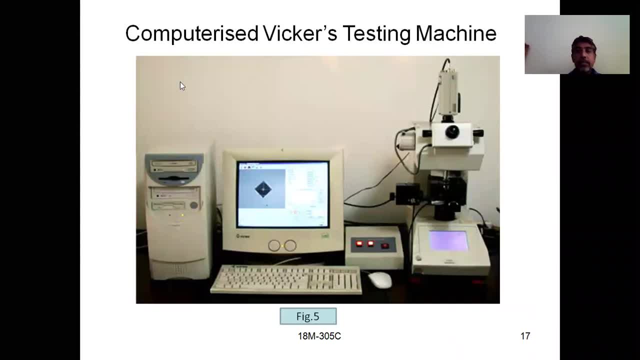 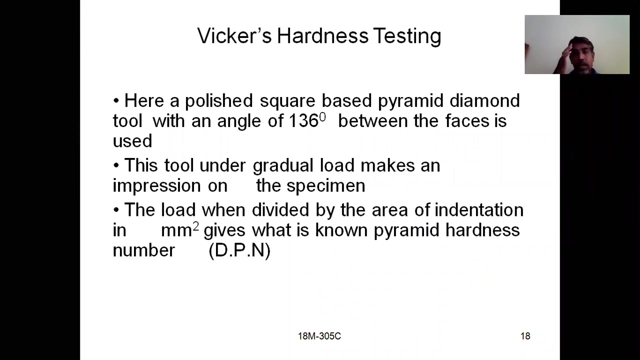 see, this is computerized vickers testing machine. if you see here, you are having a machine here and it is connected to computer. so when the test is performed here you will have a indentation and that indentation measurements can be measured here. and if you see here see what is a tool we are using and how to calculate the hardness number, if you 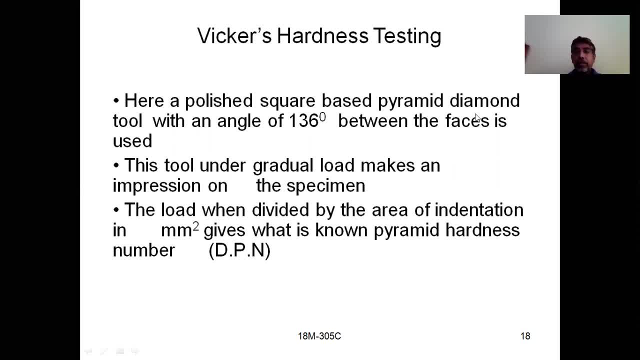 see here, here a polished, square based pyramid diamond tool. already we have discussed so which type of tool we are going to use. We are using a tool. Which type of tool we are going to use. We are using a tool of material diamond and the shape is quadrilateral pyramid, Quadriangular pyramid. we can say: 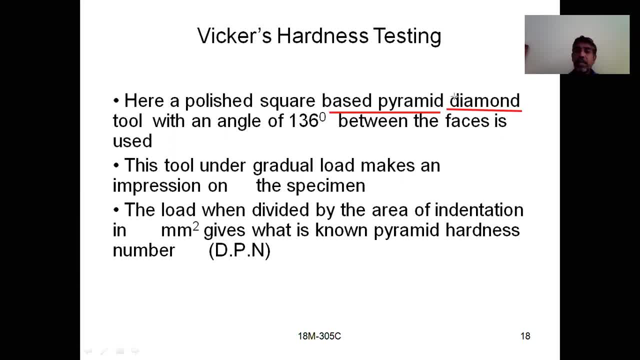 Quadriangular pyramid means you are having four faces and they are joined at a single point in the pyramid shape and the angle between the opposite faces is 136 degrees. You should remember what is the material- Diamond, What is the shape- Quadriangular pyramid- And what is the angle between the faces. It is 136 degrees. 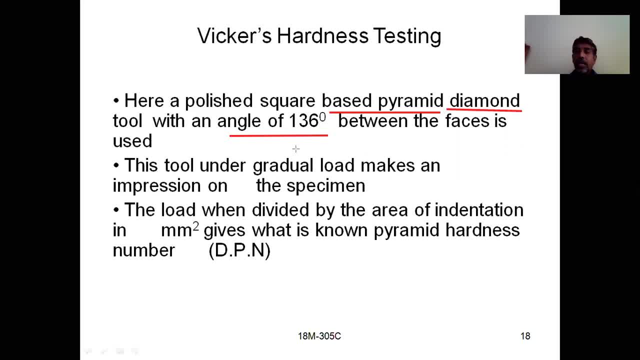 Faces means opposite faces. So how much angle between the opposite faces? It is 136 degrees. These three points we should remember while explaining. So what is the material of the indentor you are using And what is the shape of the indentor? That is nothing but quadriangular pyramid. 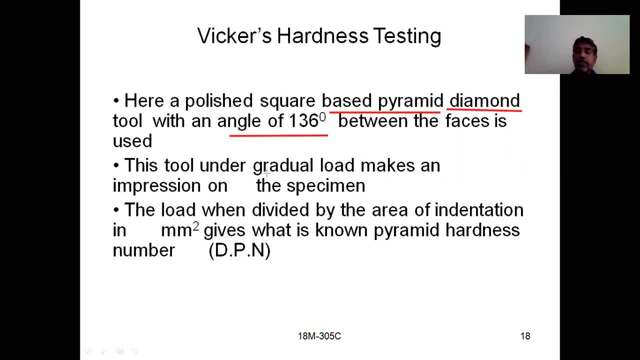 And what is the angle between the opposite faces of the pyramid? That is 136 degrees. we have to take So the tool under the gradual load and makes an impression on the specimen. So, as usual, what we have to do: First we have to touch the indentor to the specimen and later we have to apply the load. 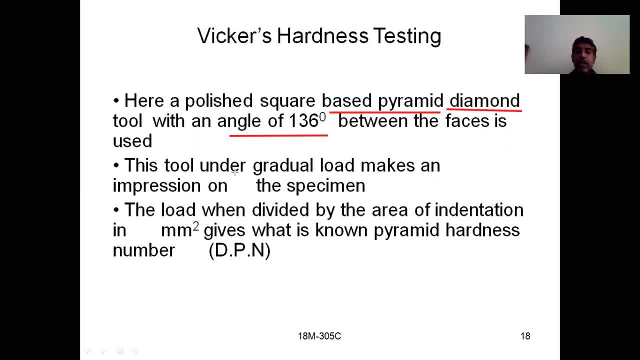 When you apply the load, what will happen? You will get some indentation. So the load should be applied gradually. That means the load should be increased slowly. So the load, when divided by the area of indentation, will give the DPM. So what you will get? You will get a pyramid hardness number when you divide the load by this area of indentation. 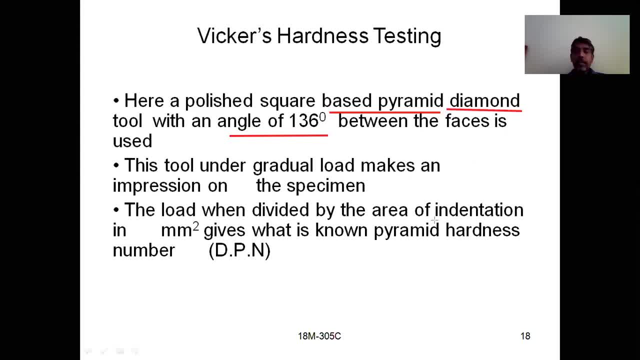 If you divide the load by area of indentation, If you divide the load by area of indentation, If you divide the load by area of indentation, you will get the DPN value. What is DPN value? DPN is nothing but pyramid hardness value. 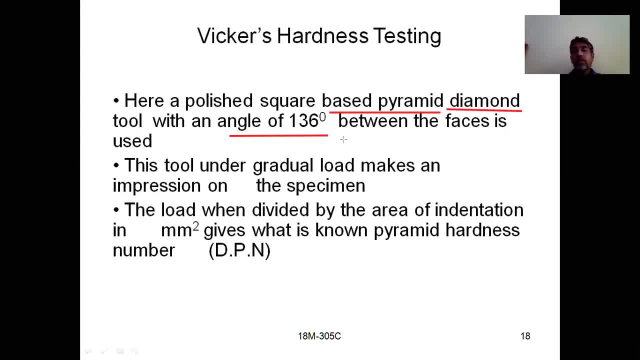 So in the Vickers hardness test we have to find out DPN value, which gives the hardness value for that material. So in this one, what we have discussed, We have discussed how to perform the test and which type of indentor we are going to use. 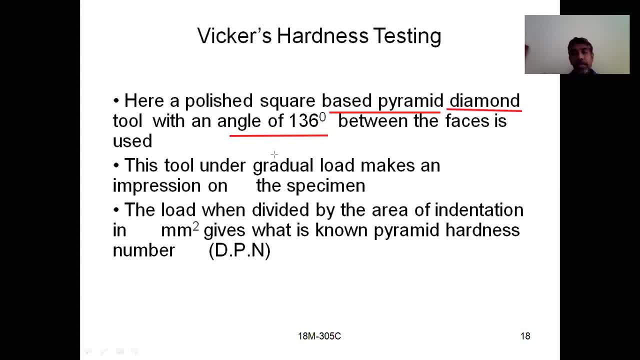 So, just you remember, We are using a diamond indentor. that is, the material is diamond, And what is the shape? It is quadrangular pyramid. What is the angle? The angle is 136 degrees between the faces, opposite faces of the pyramid. 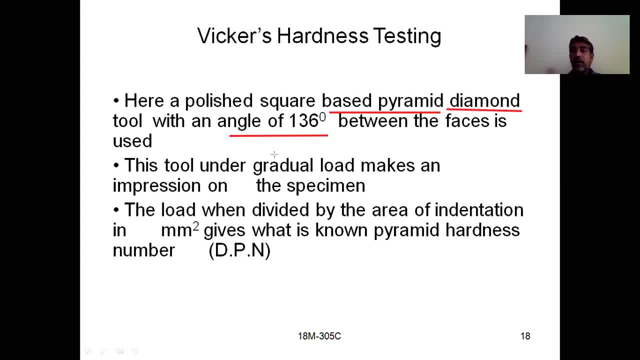 You may have surrounding faces, but we have to take the angle between the opposite faces, So that angle should be 136 degrees, And later what we have to do, We have to touch the indentor to the specimen And later we have to apply the load gradually. 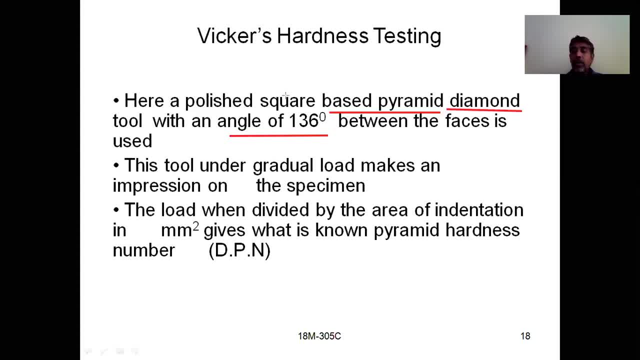 When the required load is applied, what you will get. You will get some impression. Based on that impression cross section, we have to find out the DPN value. What is the DPN value? DPN is nothing but pyramid hardness number. 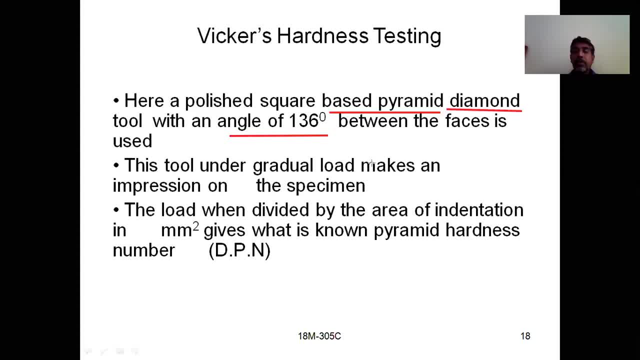 So how you will get this DPN number If you divide the load by area of cross section of the impression or your indentation. So you are getting an impression or indentation, You have to find out the area of that indentation And you are applying the load. 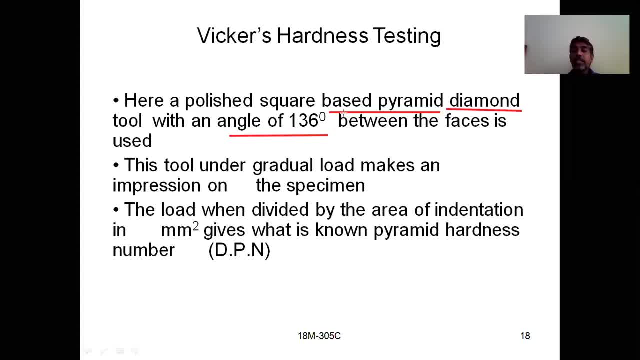 You know that load value, So that load divided by this area of indentation gives the DPN value. DPN is nothing but pyramid hardness number, So you should remember what is DPN, How to get that DPN. And coming to the next point, 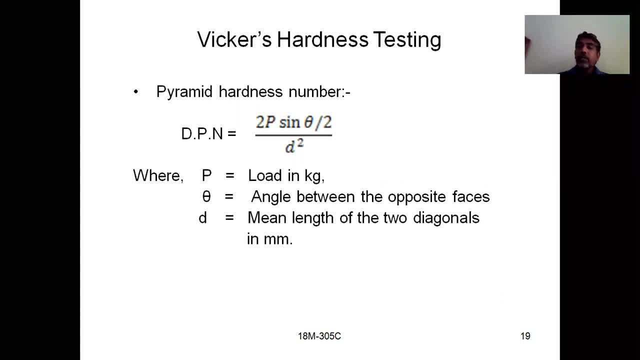 See What is the formula for DPN, How to calculate that DPN value? So by substituting the area, all these values. So what is the generalized formula for DPN? It is the load by area of indentation. So if you substitute, load is P. 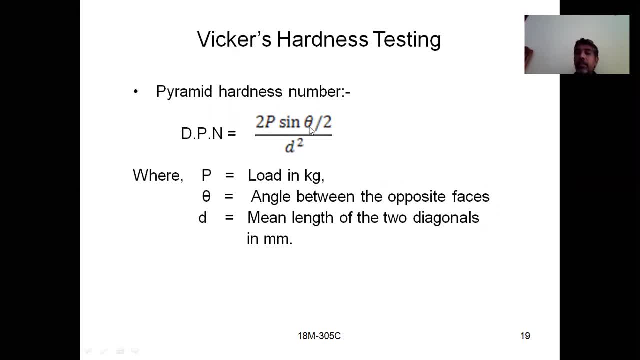 And if you find out the area where theta is from that one you will get from the indentation. Okay, So here. angle between the opposite faces, How much? It is constant, That is 136 degrees, And D, What is D? 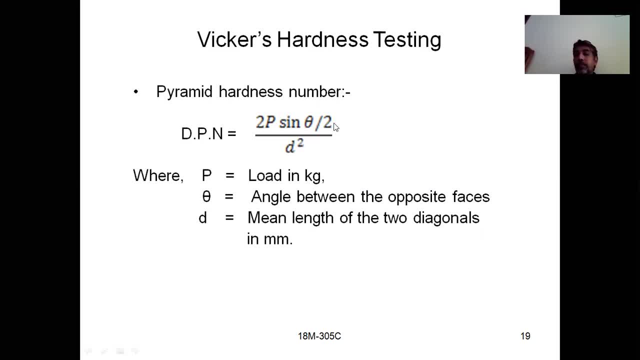 This D is the parameter here. If everything is known here, DPN, we have to find out. P is the applied force, It is known value And theta is the angle between the opposite faces. It is already fixed. That is 136 degrees. 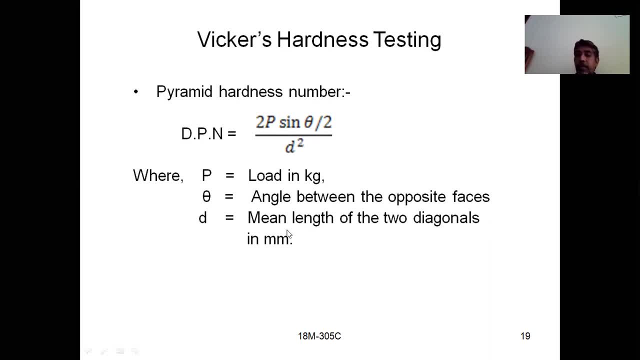 And only parameter is D. So what is D? It is nothing but Main length of the two diagonals. So main length. You are having two diagonals, So from that one you have to find out the main length of the diagonals. 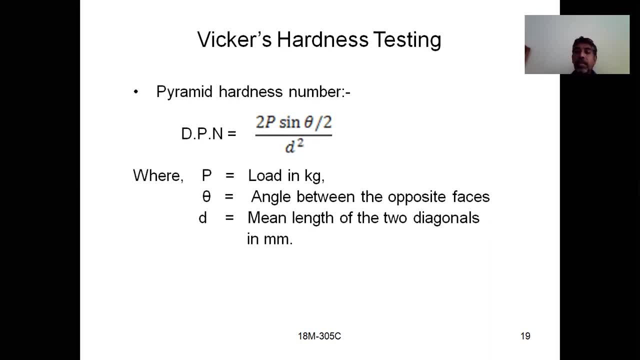 Okay, You have to take the average value of the two diagonals, Then that will become the D. If you substitute 2P sin theta by 2 by D square From this one, you will get the DPN value. Okay. So I am repeating once again. 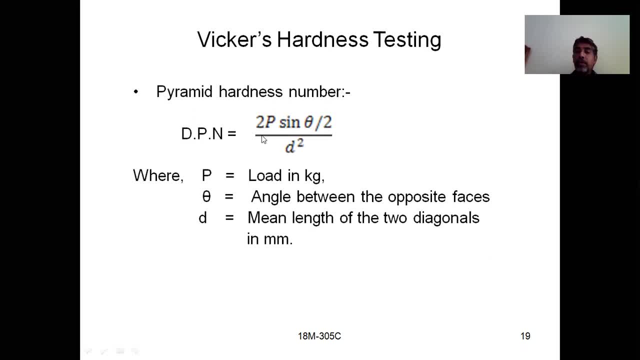 It is a very simple formula. We know that DPN is equal to Load by area of the indentation. So load is nothing but P. So how to find out the area of indentation? To find out the area of indentation, First we have to find out the 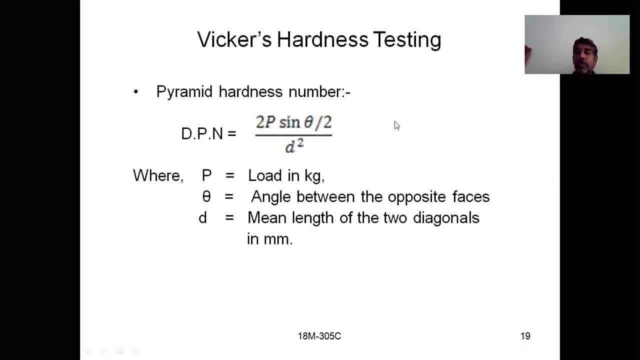 Main length of the two diagonals. So you are having two diagonals. From that one you have to find out the Main length of the diagonals And later you substitute, And that means You have to calculate the area of the indentation. 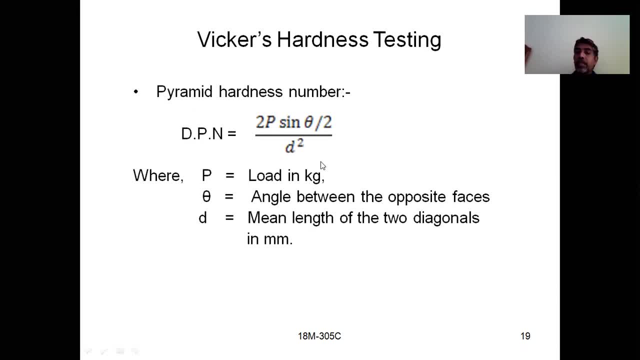 If you calculate the area of indentation, You will get this formula, That is: DPN is equal to 2P sin theta by 2 divided by D square. So in this one Everything is known Except D. This P is applied force. 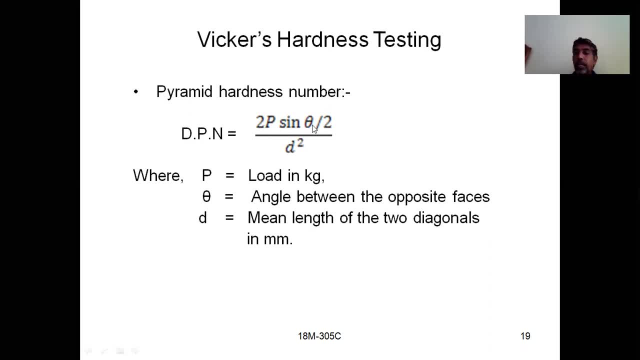 It is known, Theta is a constant, That is nothing but 136 degrees, And D is the unknown value Which we can find out from the Impression Or the indentation. If you substitute all the values in this one, You will get the. 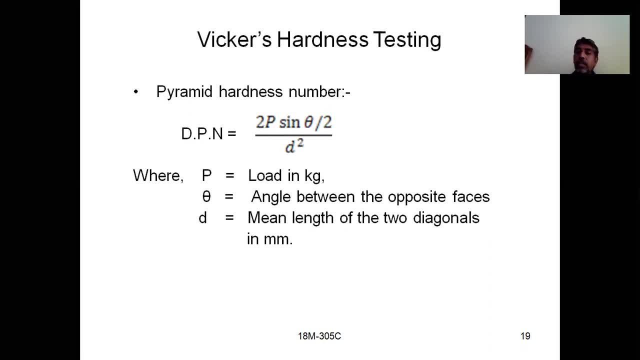 DPN value. That is nothing but Pyramid hardness number. So in this way You will find out the Pyramid hardness numbers In Vickers hardness test. Okay, So If you substitute all the values In this one, You will get the. 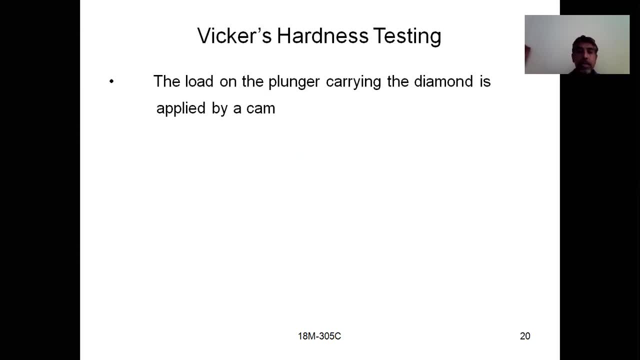 DPN value. That is nothing but Pyramid hardness number. So in this way You will find out the DPN value. If you see What, How the Load will be applied. Okay, So I already told you. 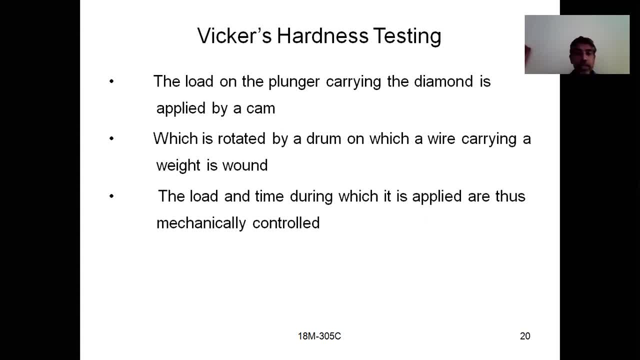 We have to apply the load Gradually. So how to apply the Load We will Discuss. So the load On the plunger Carrying the diamond Is applied by cam. So how you will apply By using a cam mechanism. 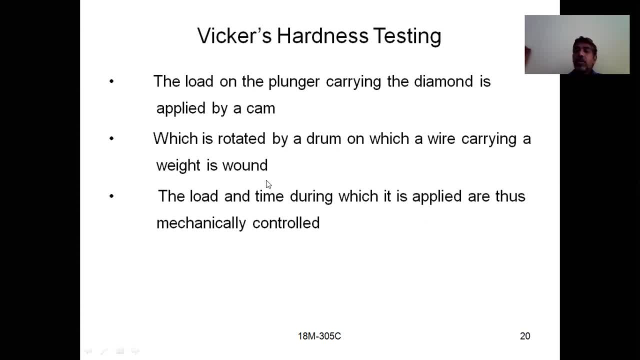 Which is Rotated by a drum On which A wire carrying Weight is wound. So Here, What we are discussing is How the load can be applied. When you apply the load Using a cam And that cam. 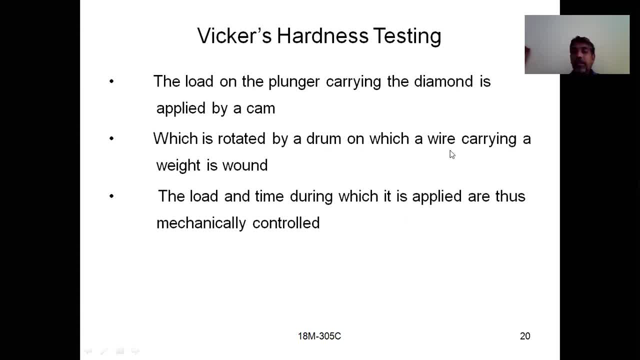 Is rotated By a drum On which You are having a Wire. For that wire You are having a weight, So the load And the time During which it is applied Is mechanically controlled. So If you see the 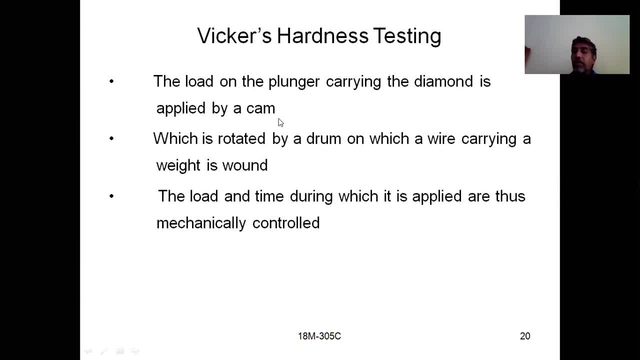 A drum And a wire Carrying a load And if you see the cam, Mechanism, Cam- All Comes under Mechanical elements. So How you are controlling the Load And the duration of the load Mechanically. 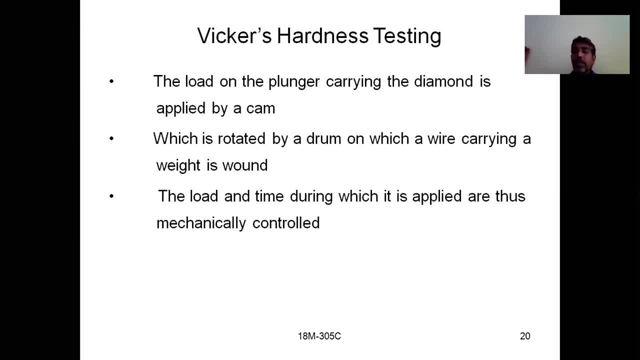 So You are using Mechanical elements here To apply the load As well as To control the load. So that's why Here you are using a Mechanical system To apply the load. Okay, This is How to apply the load. 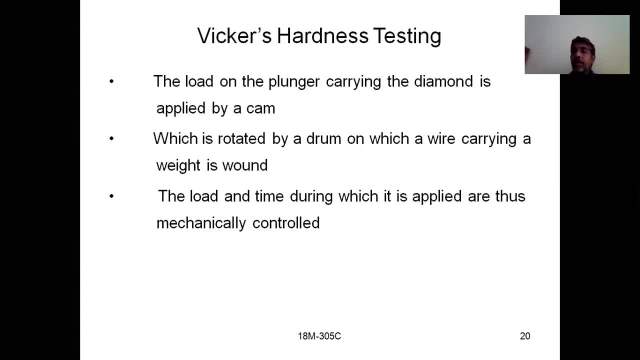 In Vickers testing. That means Which mechanism We are using Generally. So the mechanism May be vary, But the test procedure Will not vary. Here we are using Some mechanical system, Some Somewhere You may use. 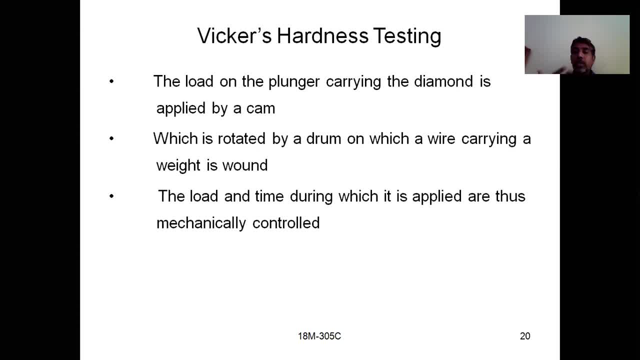 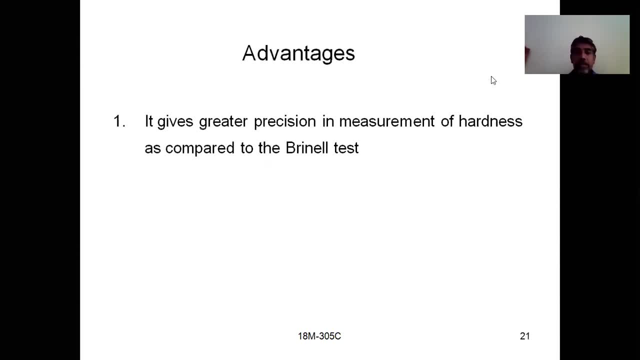 Some hydraulic system Somewhere. You use Some hydraulic system, But the mechanism Will not change. Only the mechanism For the applying Of the load Will change. And if you go For the next Slide, What are the? 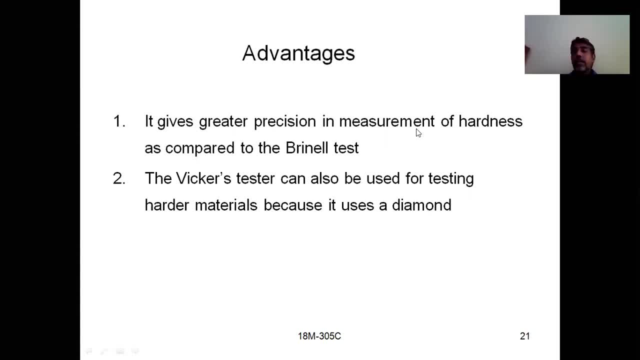 Advantage. So first We have to know The advantages. If you see, What is the advantage? Here? We can Measure More Hardness Materials. That means Hardness of Very hard Materials, Because We are using 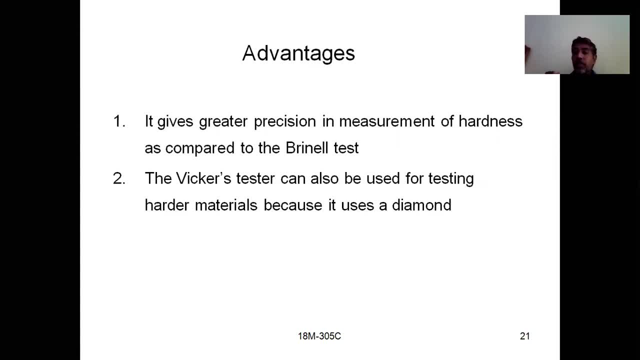 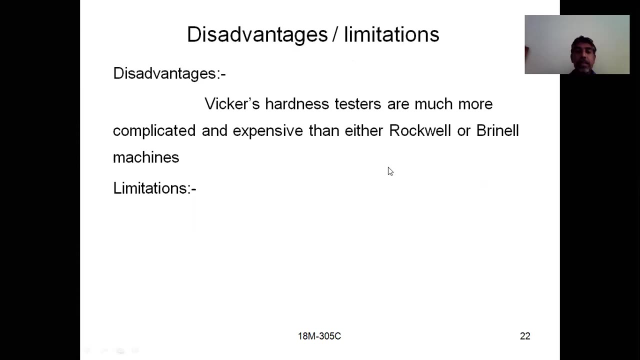 A Pyramid Type Diamond Indentor Which is Having Small Cross Section At The Edge. Okay, So Because Of That One We can Use A Smaller. 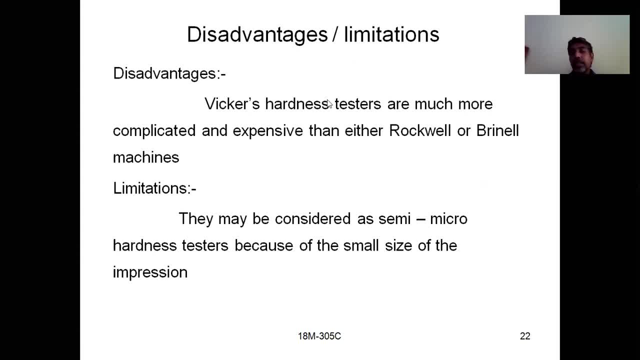 Cross Section Materials Also And Limitations. So If We Have A Hardness Test, With This Hardness Test The Cost Will Be More. Why The 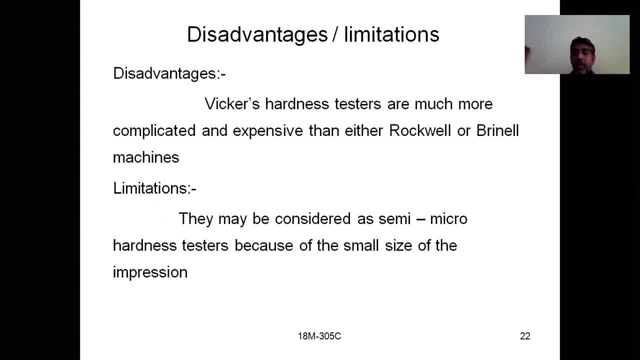 Cost Will Be More And It Is Very Complicated Because You Is Very Costly, So It Is Expensive Process. So That's Why When You 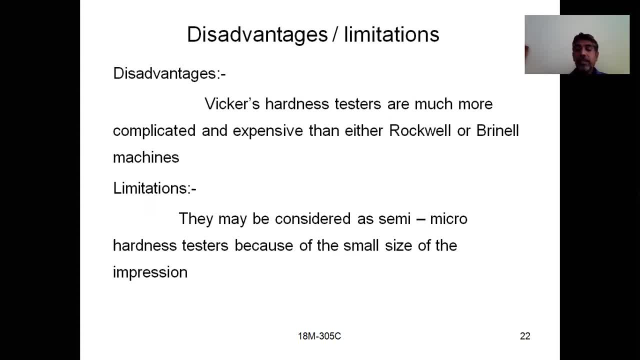 Compare With Rockwell Hardness, We Can Say That This Hardness Test Is Much Costlier. Okay, So Here You Are, Getting Small Impressions Because 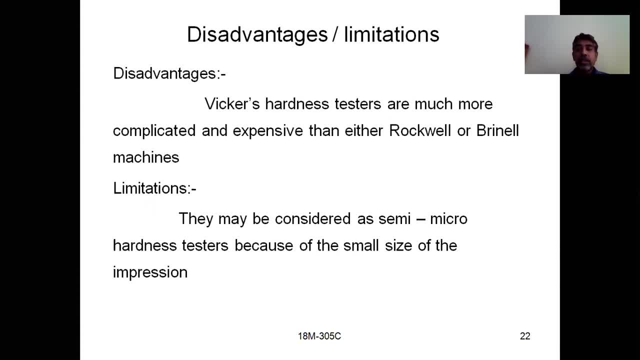 Of That One, We May Treat It As Semi Micro Hardness Test At Micro. Without Microscope We Are Unable To See Those We Have To. 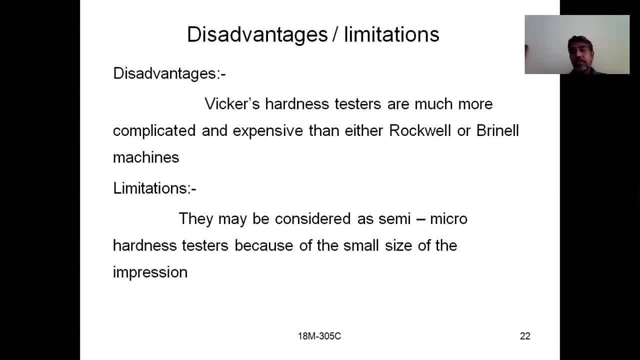 Use A Microscope. So Simply We Can See That It Is A Semi Micro Hardness Test. Okay, This Is The Disadvantages And Limitations. 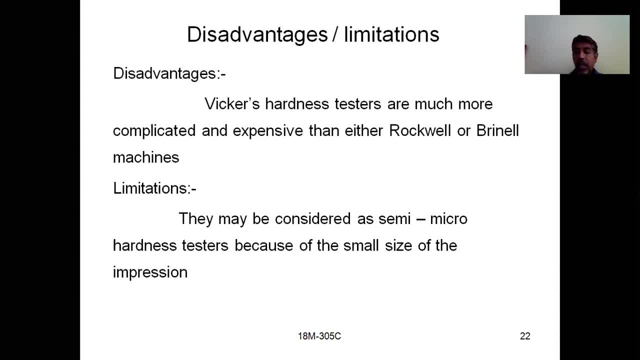 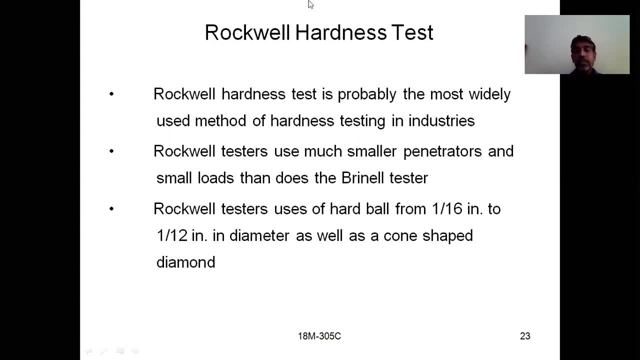 We Are Having A Hardness Test And If You Come Into The Most Important Hardness Testing Method, That Is, Rockwell Hardness Test, If You 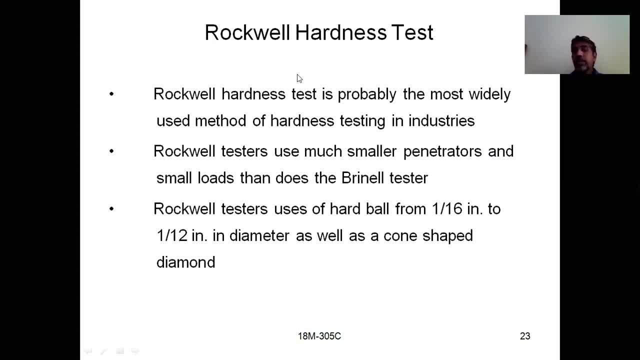 See The Rockwell Hardness Test. So This Is A Ball Intender Of One By Sixteen Inch To One By Twelve Inch And A Cone 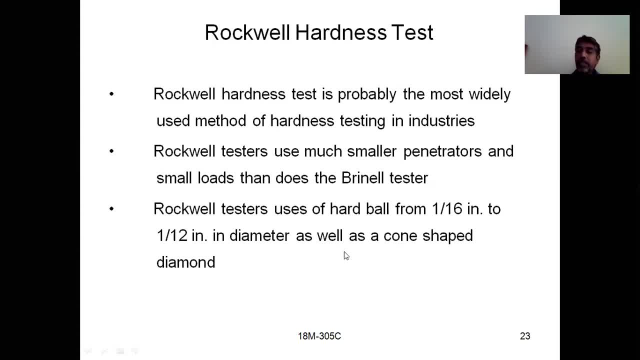 Shaped Diamond. Okay, In The Vickers Hardness You Are Using A Which Type Of Him? We Have To Remember While Explaining This, Rockwell. 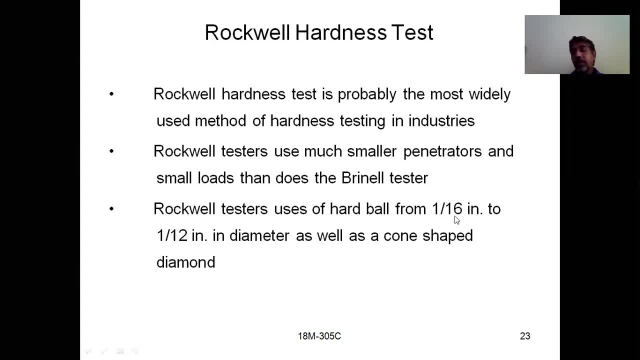 Hardness And Vickers Hardness Here. If You See The Steel Ball Also, You Are Using Very Small Size. It Is A Hardness Which Gives. 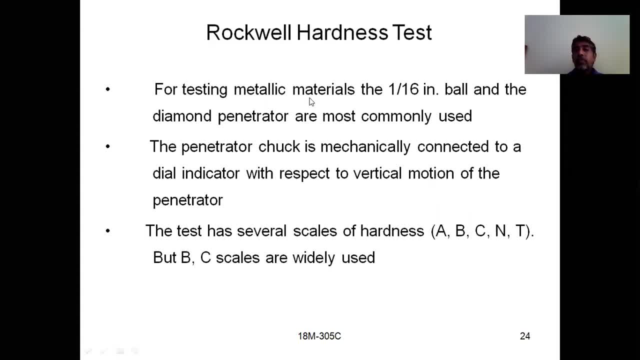 The Advantage Over Your Brinell Hardness Test And If You See Here So For Testing Of Materials, Metallic Materials Generally, We Will Use One. 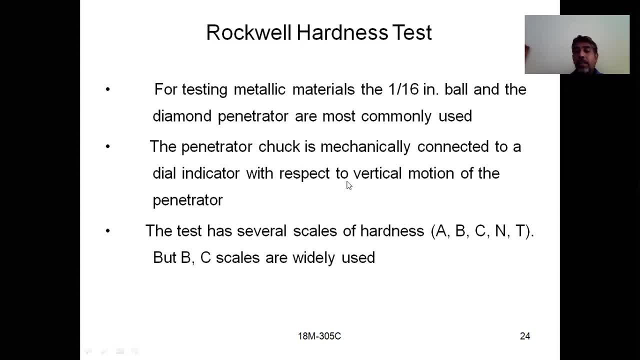 By A Steel Ball Indicator And You Can Record That Vertical Motion Of The Penetrator And The Test Has Several Scales Of Hardness. That 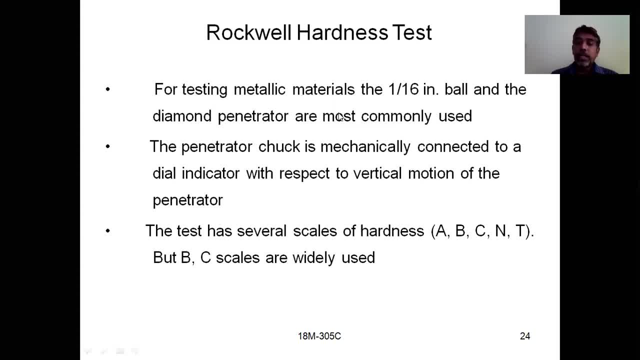 Is A, B, C, M, 19.. And Here You Are Having A Dial Gauge Which Is Connected To The Vertical Motion Of The Penetrator. 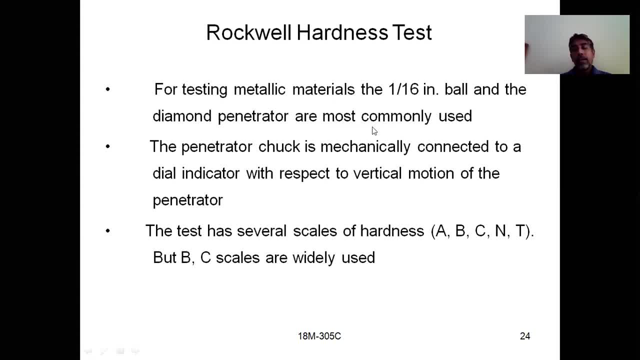 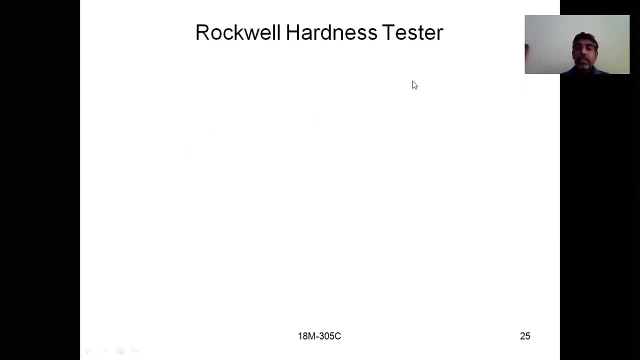 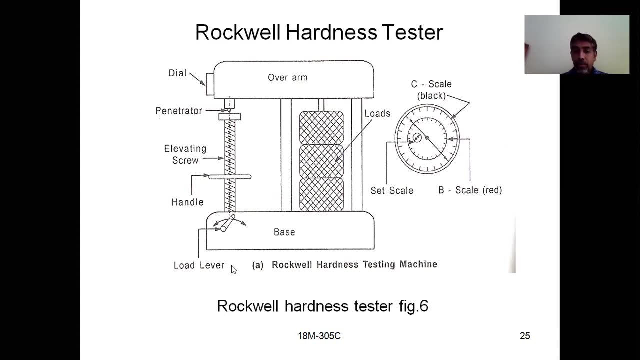 So It Can Record The Vertical Motion Of The Penetrator And The Hardness Test. So, How It Is, You Are Having A Base On. 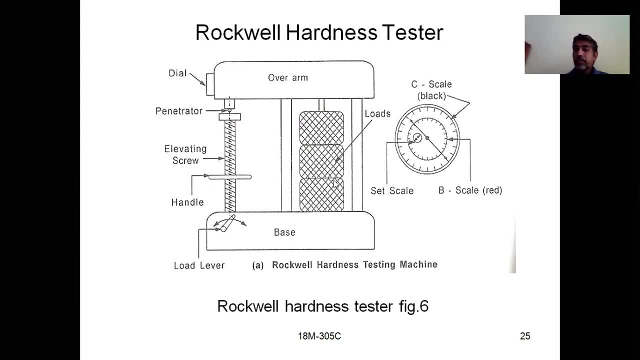 That Base You Are Having M, If You See The Loads. So You Are Having A Penetrator Or The Indentor, And Here You Are. 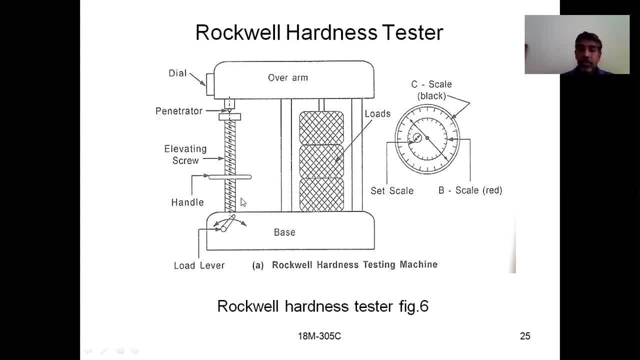 Having A Elevated Screw And That One, You Are Having An Wheel, And This Is The Hand Wheel. So For Rotating, Okay, And If You 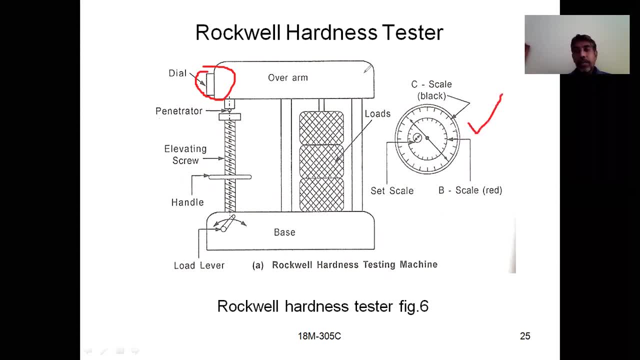 See This One And If You See This One. This Is That Scale. So How, What You Are Having, You Are Having, If You See This. 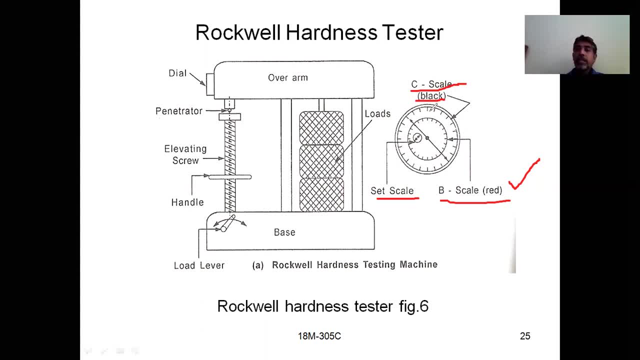 Scale Is Black. Color. Okay, So In The Complete Exams They Will Ask In The Hardness Test, The Color Of The C Scale Is Black. 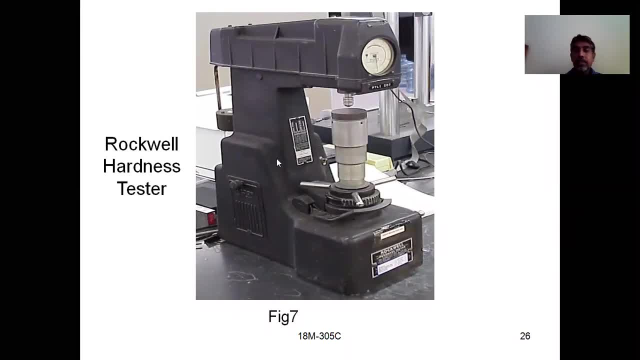 The Color Of The Hardness Test. So Just Now We Have, You Have See, Just Now You Have Observed, That Is What We Can Call. 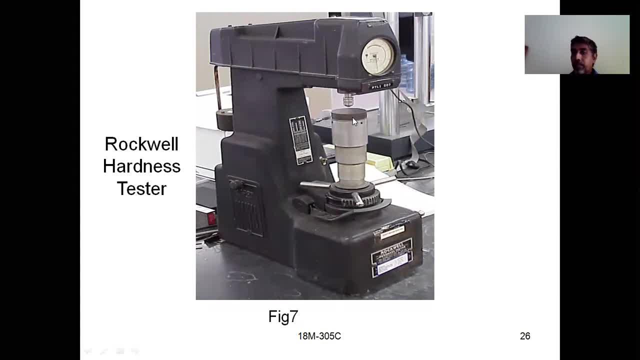 A Line Diagram, But This Is The, This Is The Indent Holder And This Is The Indent. It Is A One By Sixteen Ball. 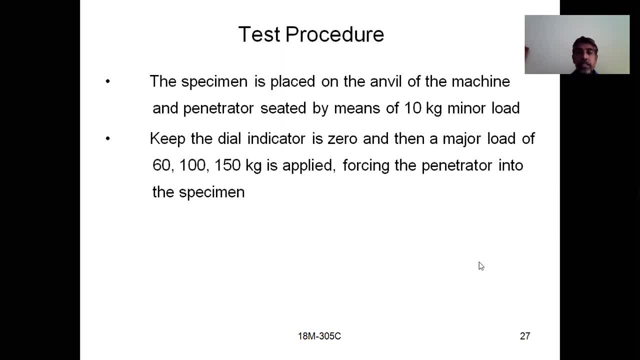 In One By Sixteen In Ball Inventor, And This Is Your Scale. So First, What We Have To Do To Remove The, If Any, Unwanted 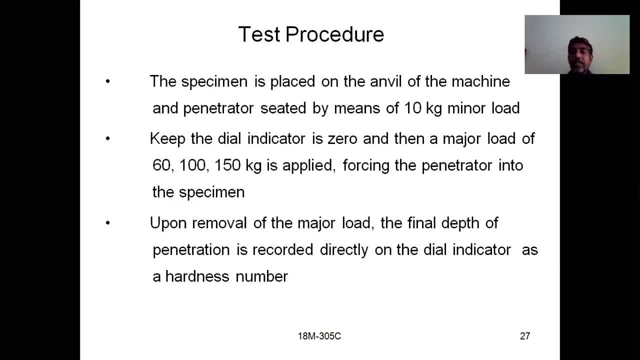 If Some Grease Or Dirt It May Be, Even Though If You Clean That One You Have The Indentor To Penetrate Into Some. 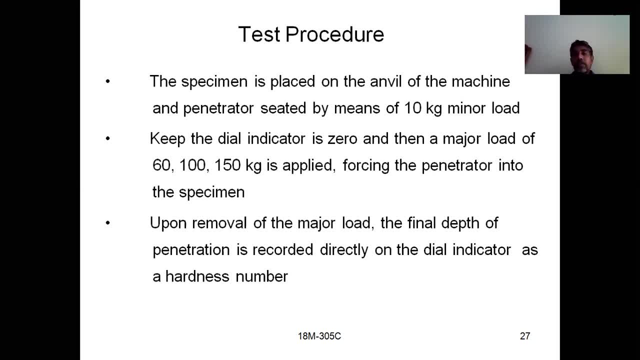 Extent And It Will Seeds Into The Specimen. So First, What We Have To Do: You Have To Clean The Specimen And You Have 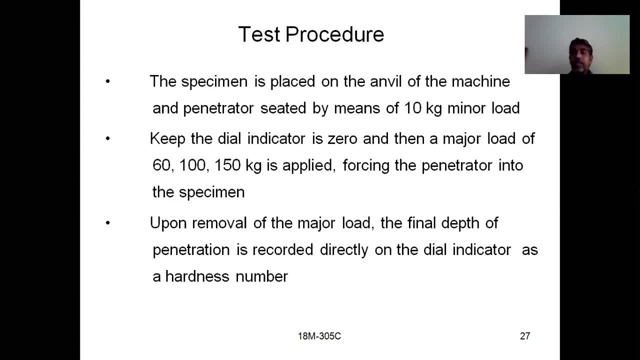 To Set The Specimen To Certain Depth. That Means It Is A Seating And Later What We Have To Do. So Keep The Dial Indicator. 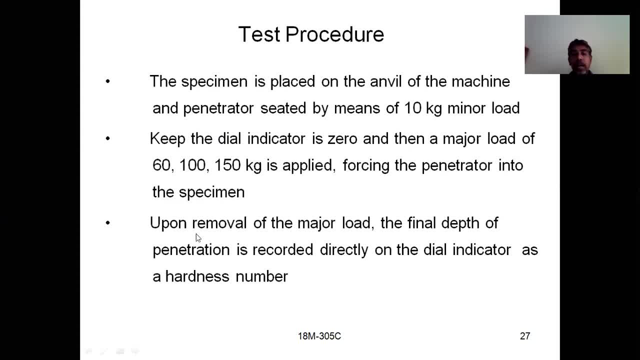 Is Zero Into The Specimen Upon The Removal Of The Measure Load, The Final Depth Of The Penetration Recorded. So Later What We Have To 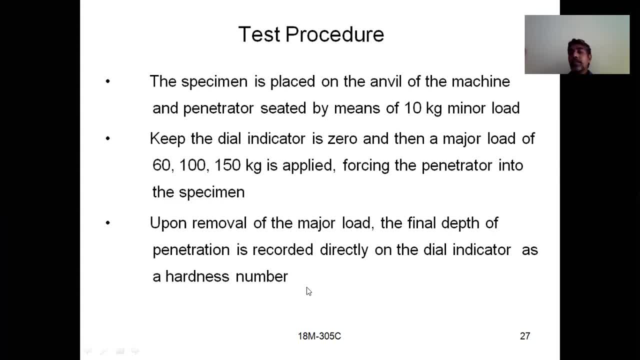 Do We Have To Remove The Test Procedure? I'm Repeating Once Again. So First, What We Have To Do: We Have To Keep The Specimen. 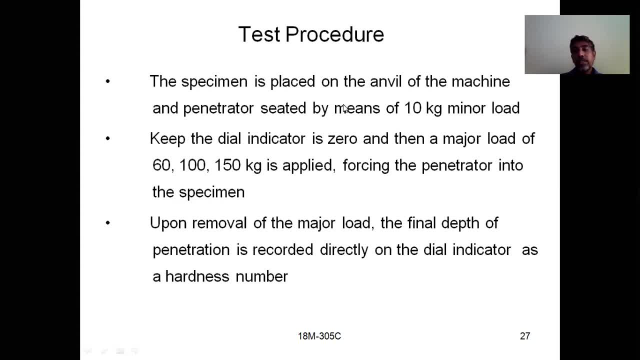 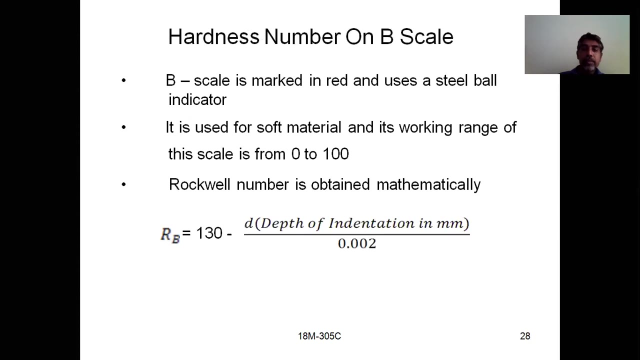 Onto The Anvil And We Have To Rotate The Hand So To Remove The Measure Load. We Have To Find Out The Depth Of Penetration. 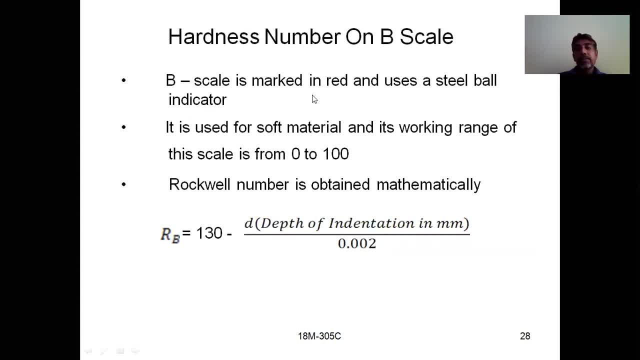 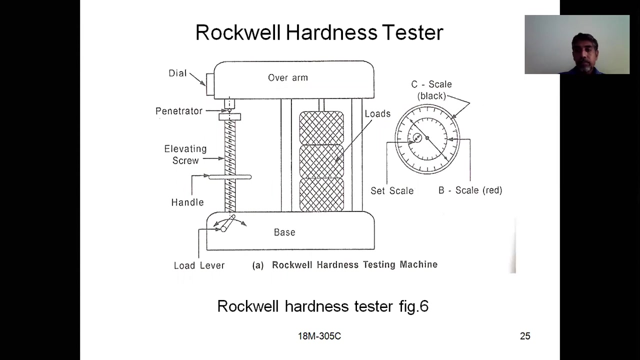 Which Is Directly. We Will Get The Harness Value From The Dial Indicator. So What Is The Color Of B Scale? It Is Nothing But. 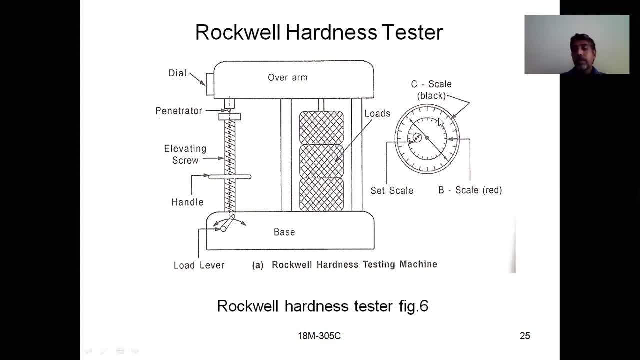 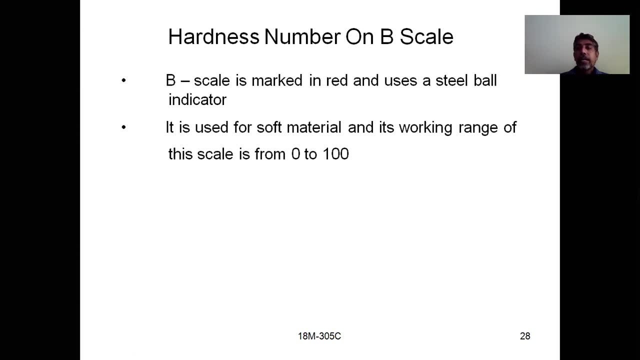 Red, If You See Here. See Here: B Scale Is Red, C Scale Is Black. So B Scale Is Used For Soft Materials And Working Range. 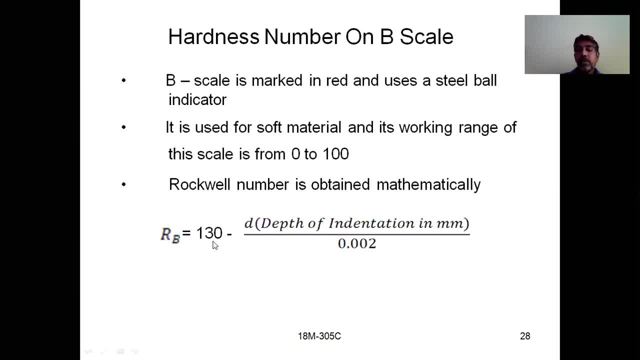 Will Be 0. To 100.. And Rockwell Number Is Obtained Mathematically By This: You By Using This Value. So What Is The Type? 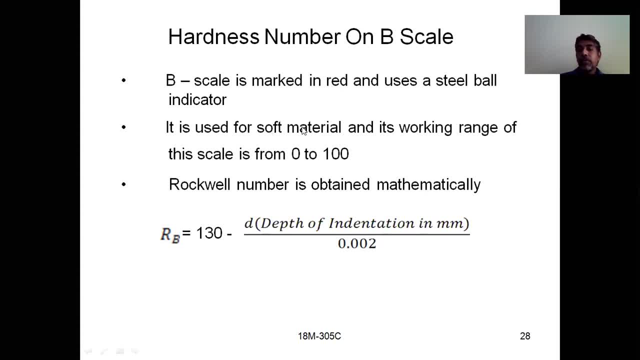 Of Indentor Will Be Used Steel Ball Indentor And For Which Materials It Can Be Used- Soft Materials. What Is The Working Range? 0.. 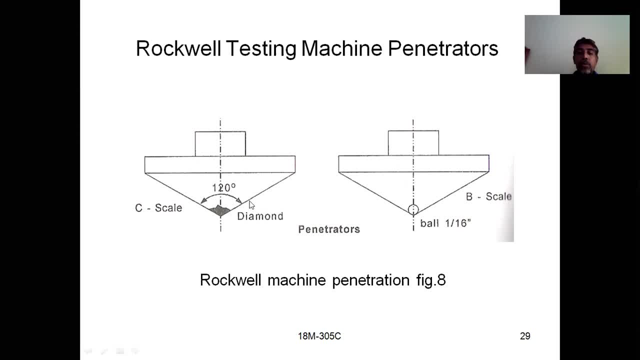 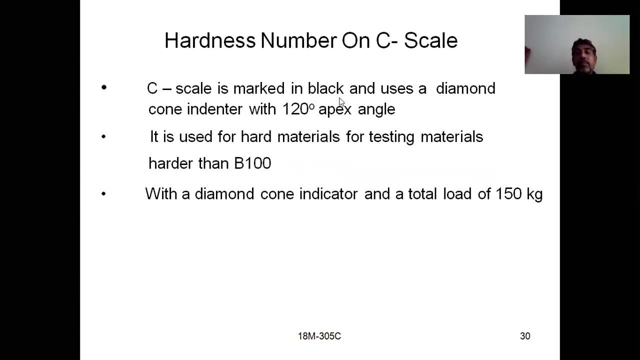 To 100.. And How Is Used For Testing Hard Materials, For Testing Harder Than B 100.. So Which Type? What Is The Color Of? 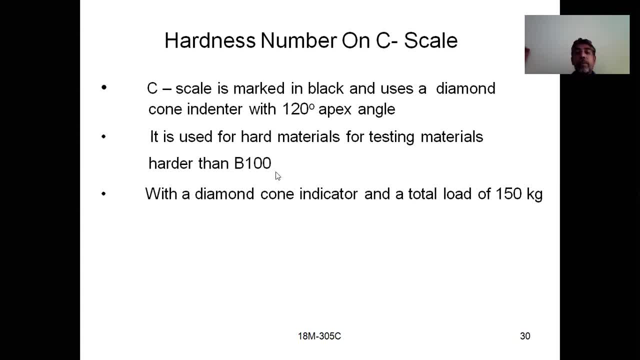 C Scale Black, And Which Type Of Indentor Used- Diamond Cone Indentor- And How Much Angle, Apex Angle 120. Degrees, And For Which? 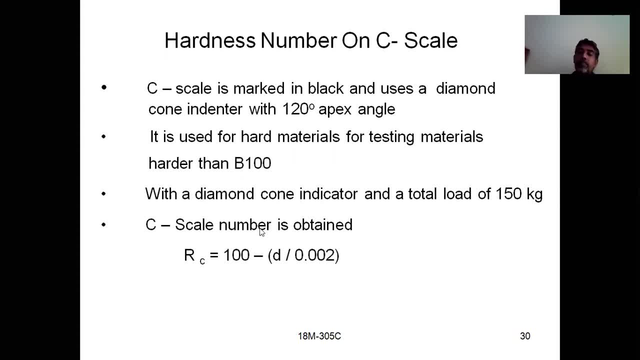 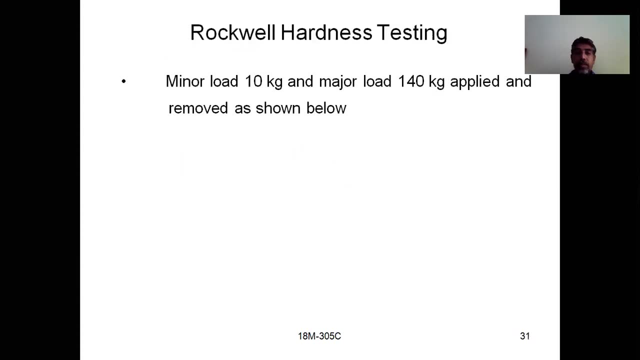 Materials. It Can Be Used Harder Materials. And What Is The Range? More Than C Scale? See Here Minor Load Of 10. Kg And Major. 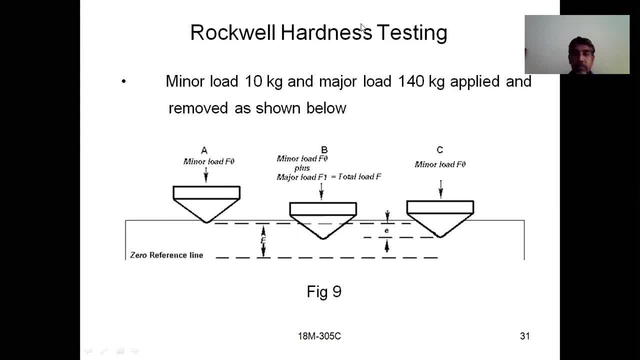 Load Of 150. Kg Applied And Removed Ash One Below, If You See Here. So This Is Your Major Load Here, Okay, So Major Load. 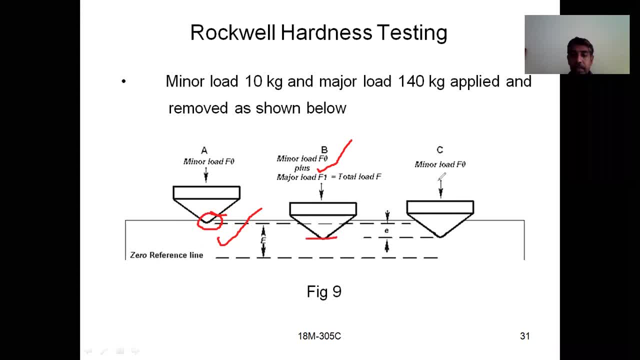 Total It Will Become This Plus This. So It Is Penetrated Up To This Level And Later. If You See Here, When You Apply The 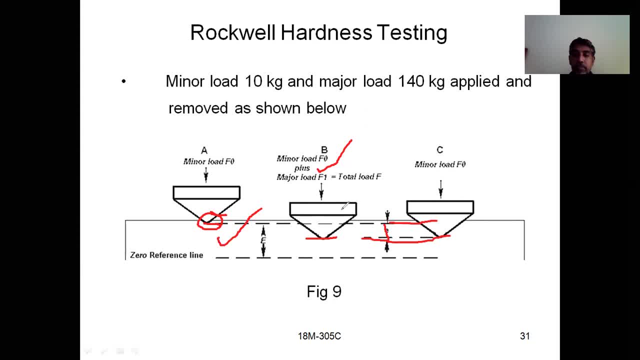 Total Load And The Penetration When You Apply The Minor Load. So This Minus Will. This Gives The When You Apply The Major Load. So 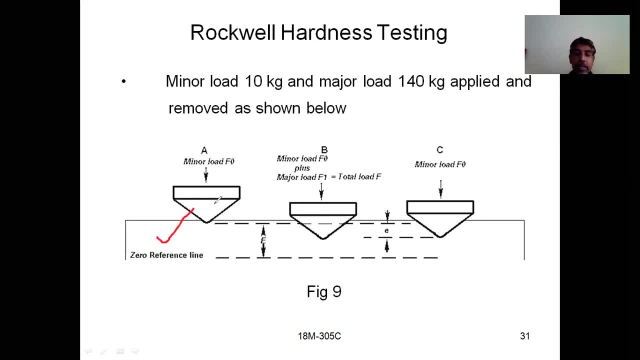 I'm. You Have To Apply A Minor Load, A Minor Load Of 10. Kg, And What Will Happen? This Inventor Will Penetrate Into 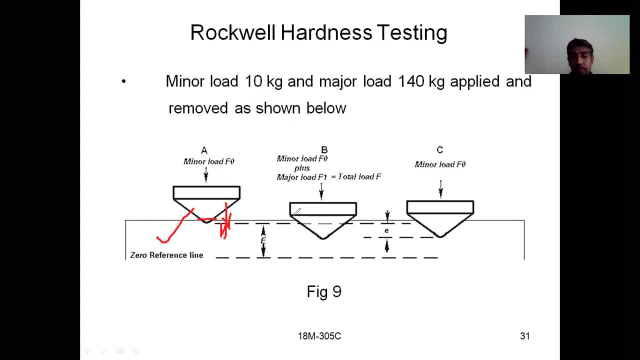 To Some Depth. This Depth, See, This Is The Major Load. Because Of This Total Load, What Is Happening? The Inventor Is Penetrating To 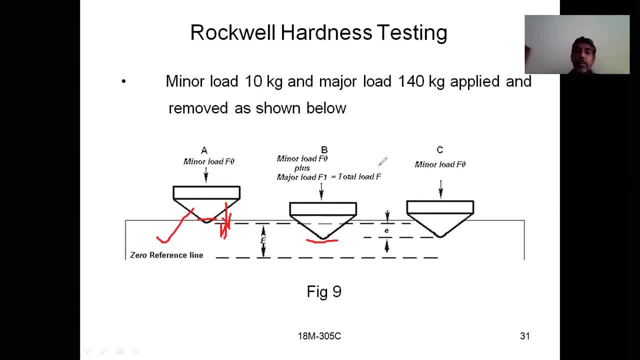 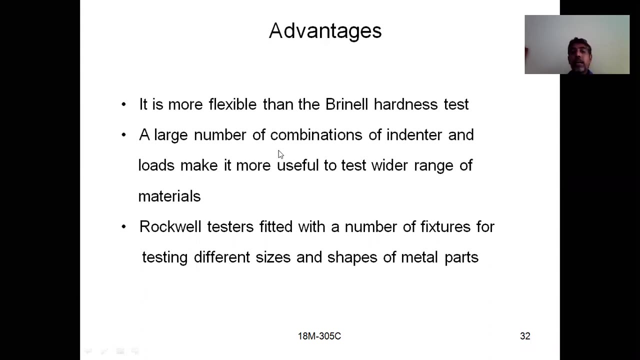 This One, This Much, And You Are Removing The Major Load And If You Do This, This Is More Flexible Than Hardness Test And Large. 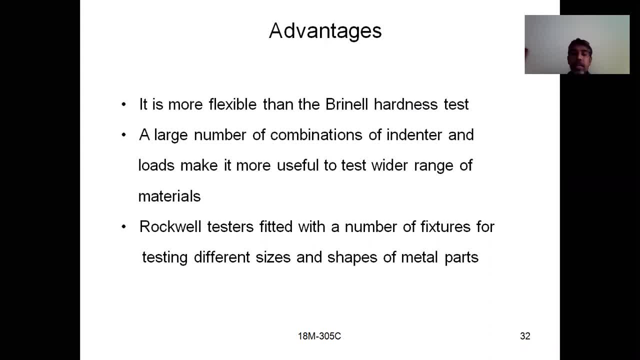 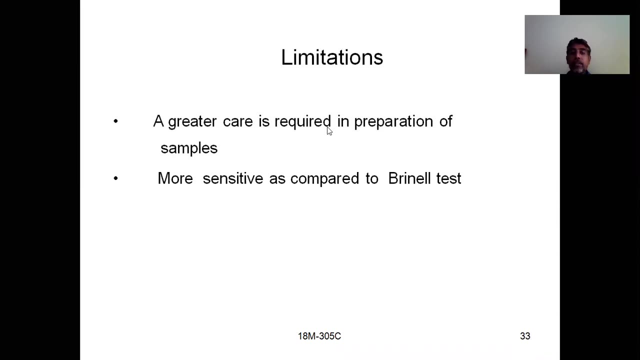 Number Of Combination Of Inventors We Can Have, And It Is Useful Test Wide Range Of Materials Because Of Samples, So Samples Should Be Prepared. 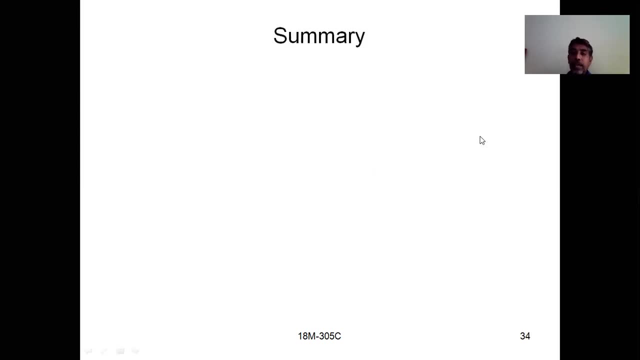 Properly And More Sensitive As Compared To Brinell Test And The Sensitiveness Is More In This Test Compared To Your Brinell Hardness. 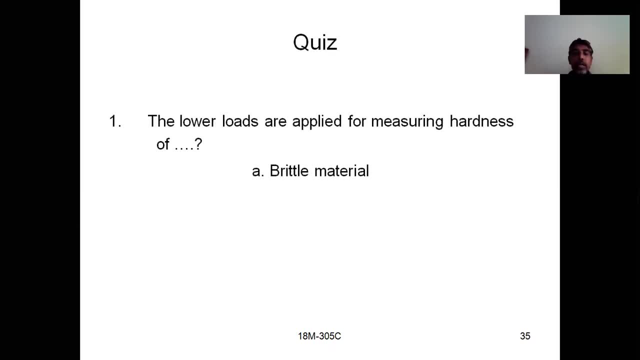 Till Now, And If You Go For A Small Quiz Here, If You Go For The Small Quiz Here, So The Lower Loads Are Applied For. 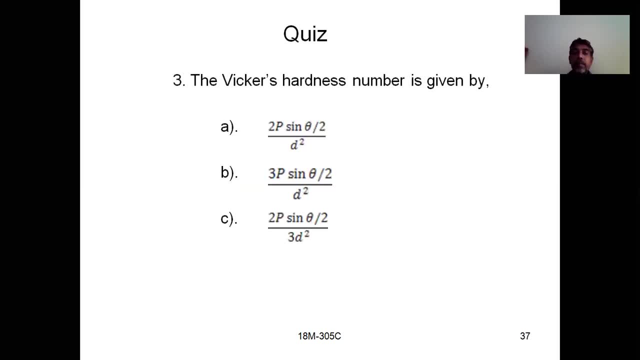 Measuring Hardness Of Hardness Is Given By 2p, Sin Theta By 2. Divided By D Square, And The Testing Machine Uses A. 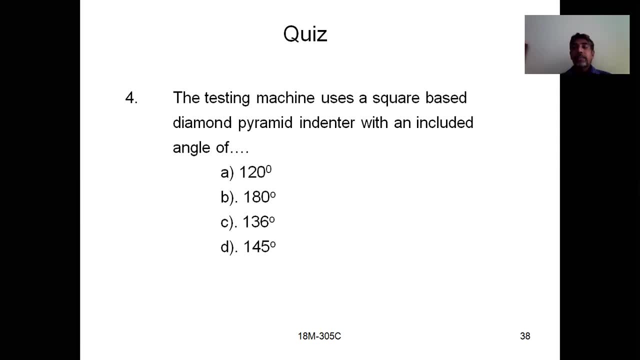 Square Based Diamond Pyramid Indentor With An Included Angle Of Diamond Which Is Used In Hardness Will Be Is 136. Degrees B Scale Uses. 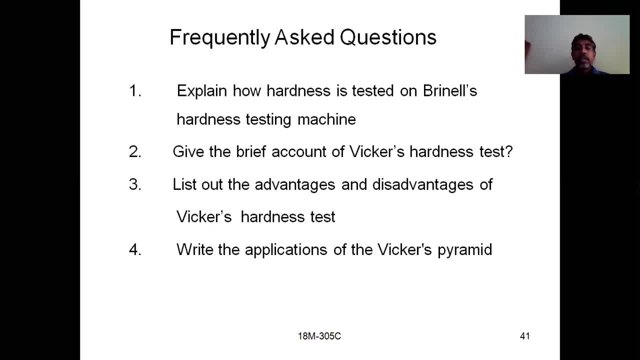 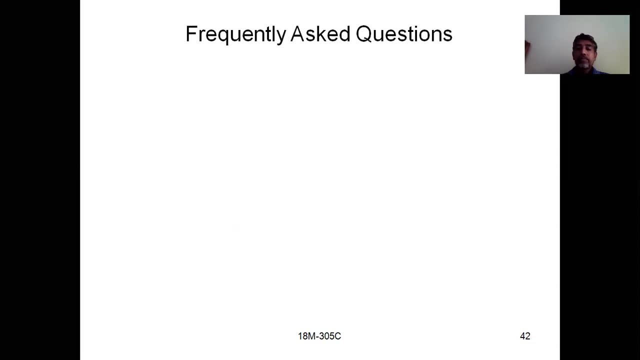 A Ball Indentor. Steel Ball Indentor. Which Type Of Scales Are Widely Used Behind C Scale And The Distinguished Between B Scale? 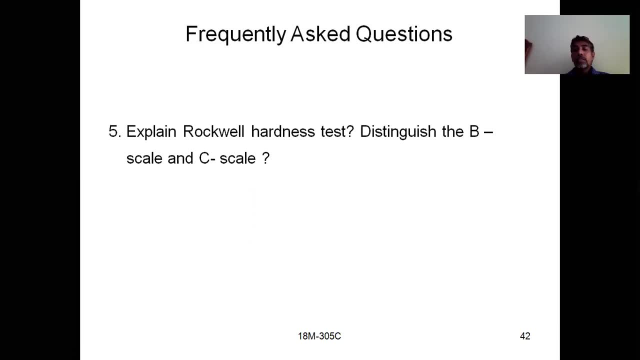 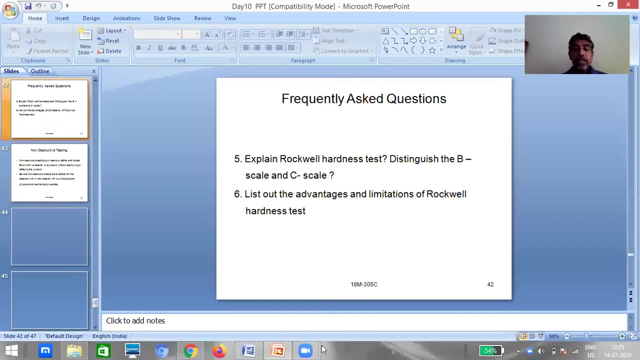 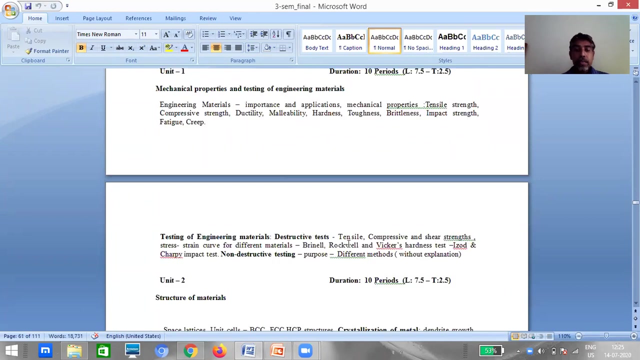 And C Scale. So What Is The Difference Between B Scale And C Scale And List Of The Advantages And Limitations Of The C Scale. 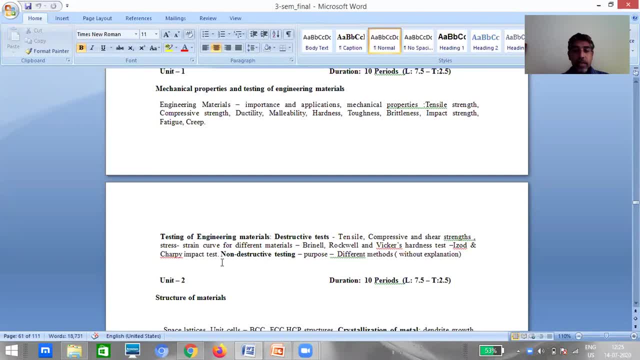 So We Have Completed This Non Districtive Testing Methods And We Are Having Non Districtive Testing Here. We Are Having Explanation Of Those Methods Only. 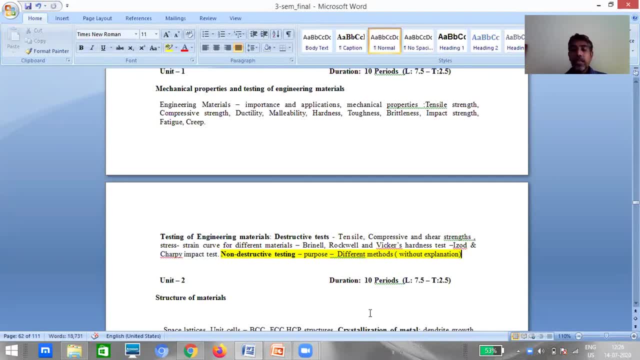 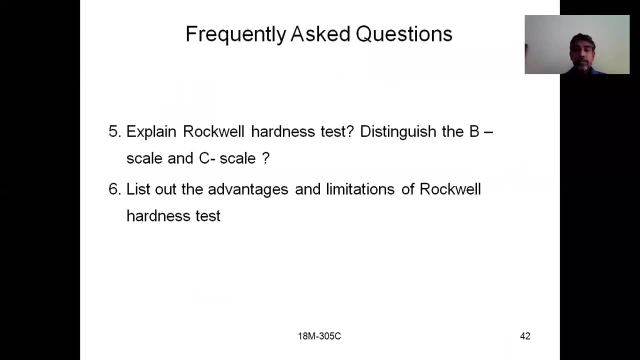 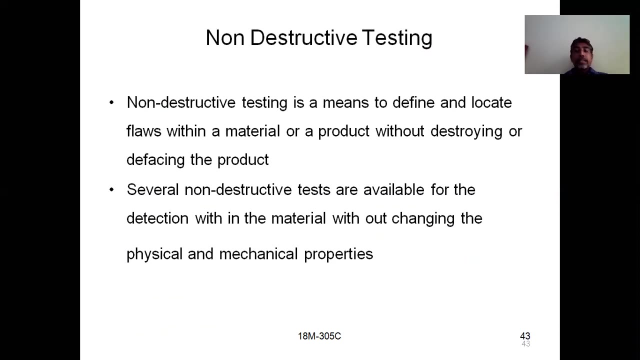 Introduction, Just Introduction, To The Non Districtive Testing. So We Will Discuss Those Things Here. See What Is Made By Non Districtive Testing, What Is? 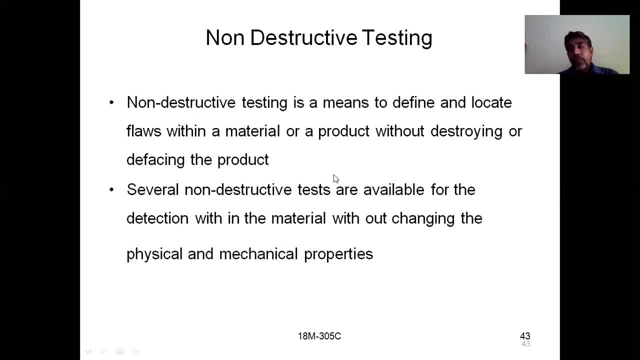 Made By Non Districtive Testing. In The First Sessions Of This Testing Procedures, In The, We Have Discussed What Is The Difference Between A Districtive 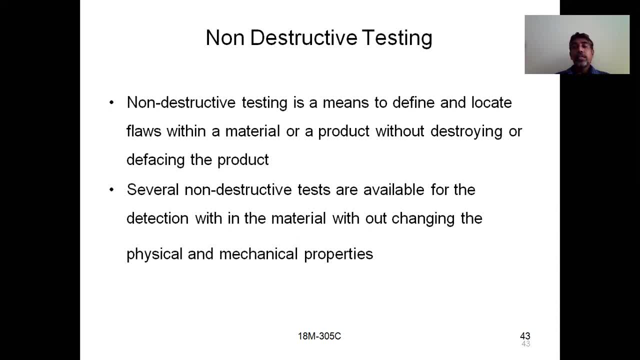 Testing And Non Districtive Testing. Okay, So We Have This Non Districtive Testing, But What About This Non Districtive Testing Without Destruction Of The? 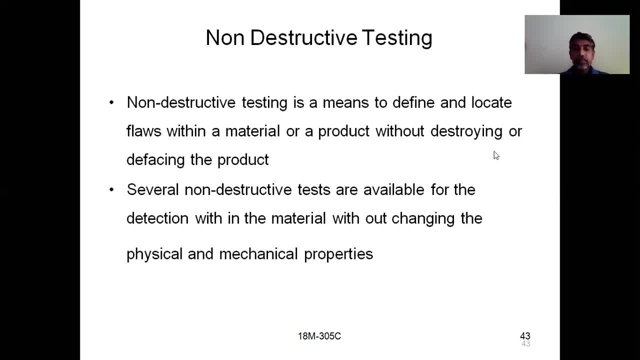 Component, We Are Going To Find Out The Faults In It. That Means Any Fracturing. Without Fracturing, Destroying Or Defacing Are Same. 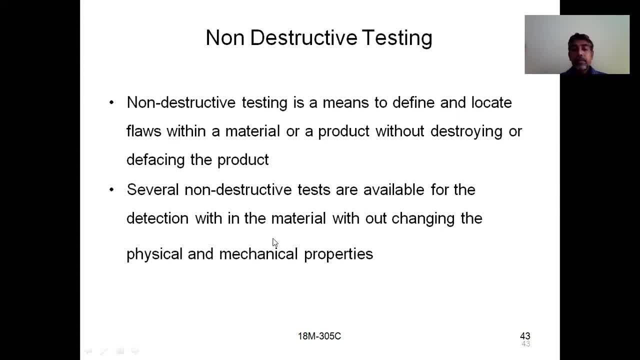 Same Meaning. Okay And Several Non Districtives Are Available For The Detection Of The Detection Of The Material, Without Changing The Component. We Are Not. 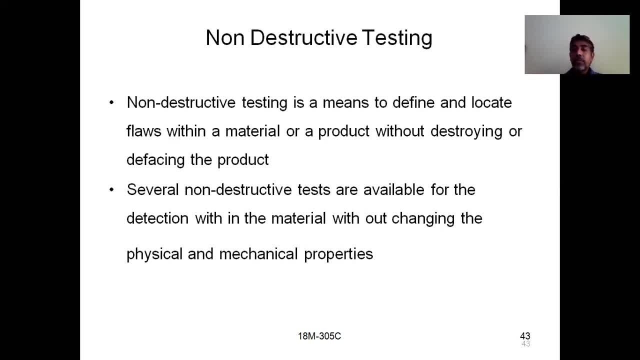 Going To Fracture Them, We Are Not Going To Break Them, We Are Not Going To Destroy Them. So, Without Destruction, We Are Going To. 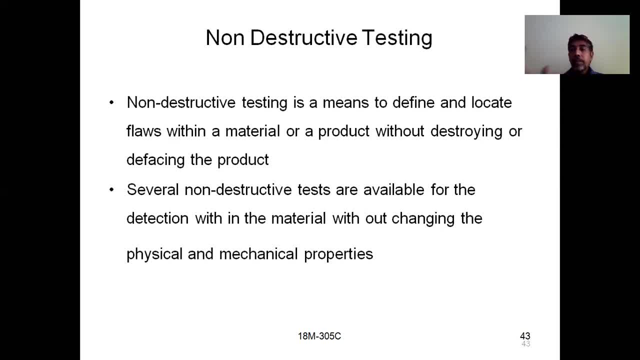 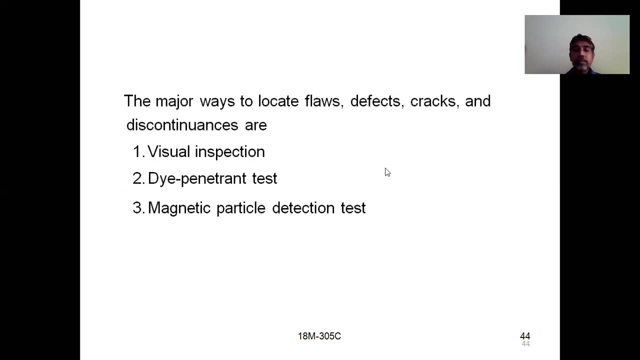 Find The Components. So What Is The Main Purpose? To Find Out The Defects In The Components Without Distraction. We Are Going To Find. 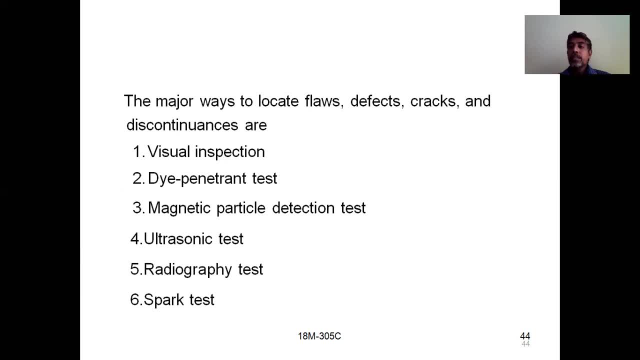 Out. So That Is The Main Purpose Is Here. We Are Not Going To Destruct Any Component Without Destruction. Also, We Are Going To Find 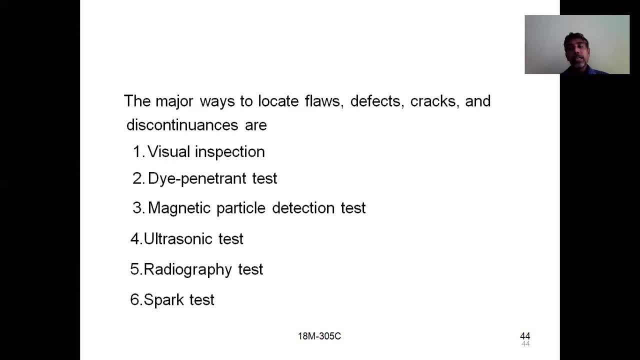 Out The Defects That Are Present, Whether It Is Distraction, Those Both Can Be. That Means Surface As Well As Internal Defects Can. 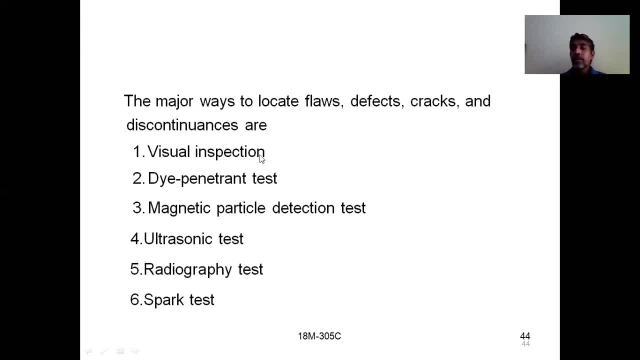 Be Found Out Here. So What Are The? If You See Here What We Are Going To Find Out, Any Component Of The Defects Also. 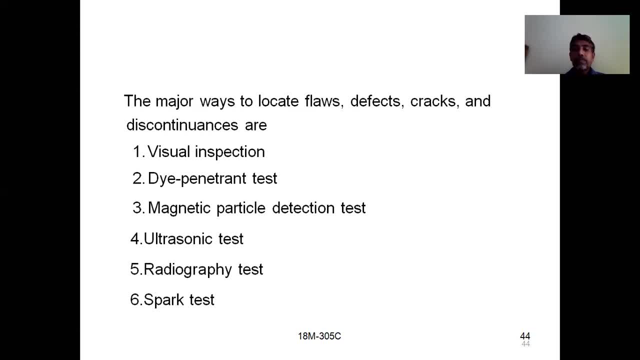 Can Find Out Any Defects. Those Can Be Found, As In The Surface Of The Defects Can Be Found. Any Defects Of The 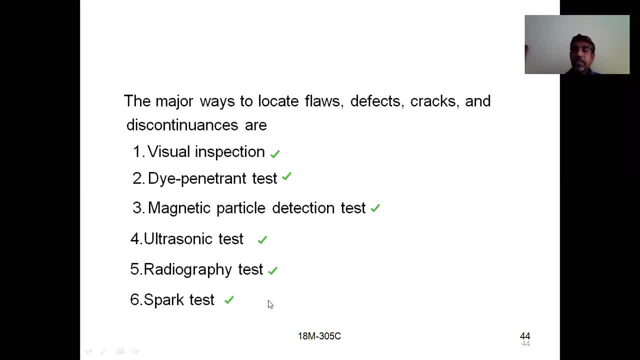 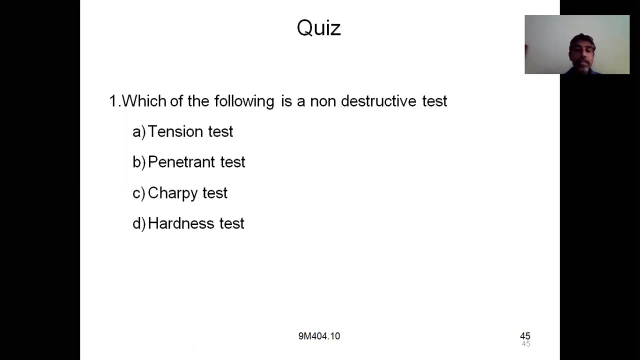 Component. So We Will Find Out The Defects In The Components. So, Based On This One, We Will See Some Quiz, Which Is The Following: 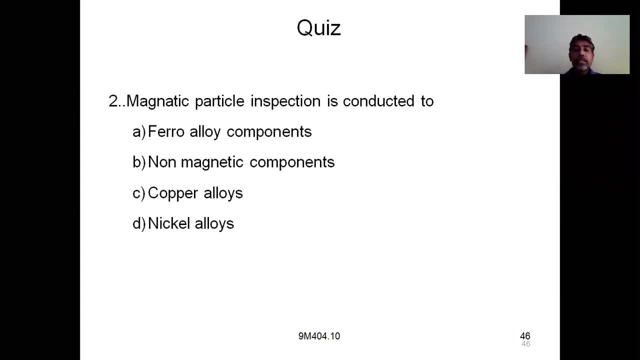 Magnetic Particle Inspection Is Conducted To Ferro Like Components, Non Magnetic Components, Copper Allies, Nickel Allies. Which Is The Answer? See Here The Limitation. 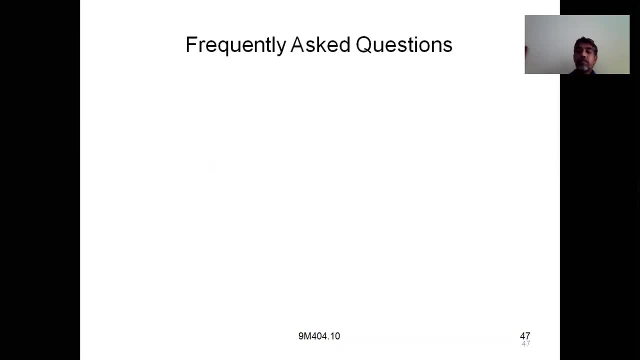 For A Magnetic Particle Inspection, The Components Of The Magnetic Components. What Is A Grand? That Is It Not. A This Is Cannot, Which Assimilate. 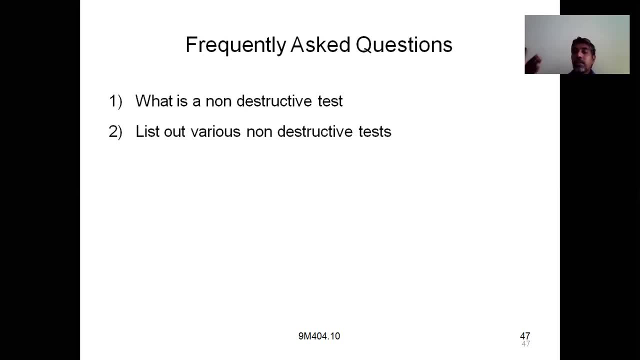 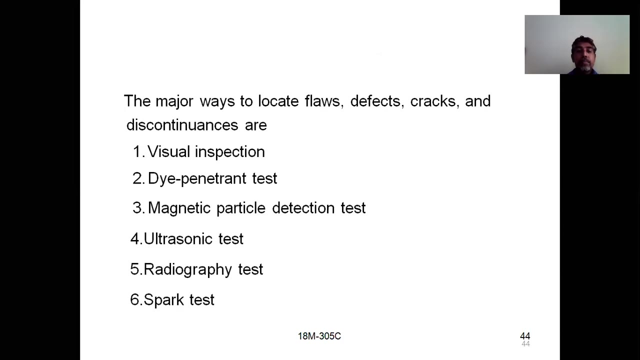 Number To The íamos Of The Magnetic Particle Of non-destructive test. see here. what are those non-destructive test we are having here? I will show you once again because it is very, very important: visual inspection, dipenitent test, magnetic particle detection test, ultrasonic test. 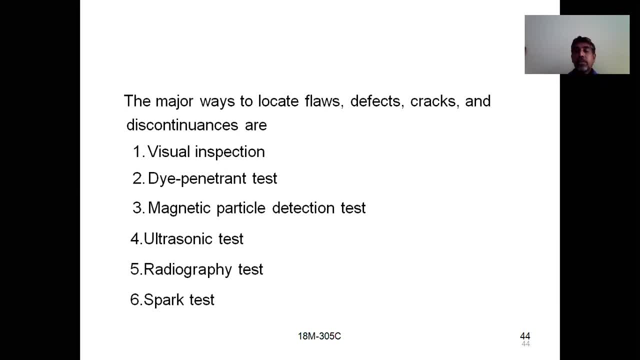 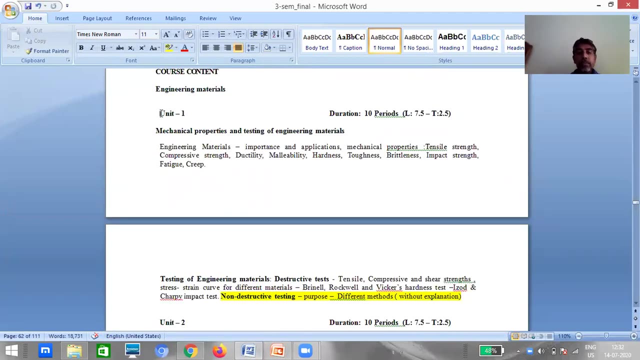 radiography test and spark test. okay, so with this one, what we have did is we have completed the first unit, so just, we will go for the syllabus, what we have discussed till now. see if you take the unit one: if you take the unit one, what? 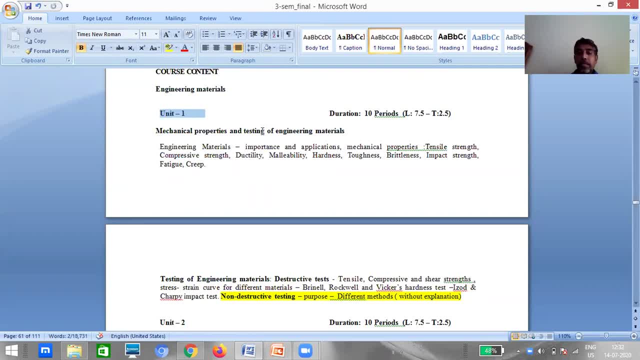 you are having in that one. you are, we are having mechanical properties and testing of engineering materials in that one. so, from the first decision onwards, what we have discussed, if you see here in the first decision, we have discussed what is meant by engineering materials and what is the importance of engineering. 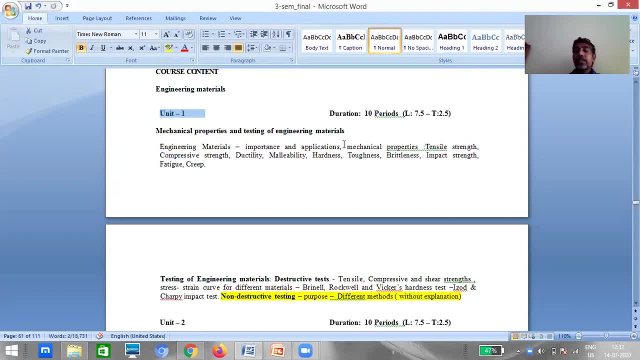 materials and what is the classification of engineering materials and what are the applications of engineering materials. we have discussed later. we have discussed the property spectrum and in that one, for a mechanical engineers the mechanical properties are very, very important. and we have discussed mechanical properties, so we have discussed tensile strength, compressive. 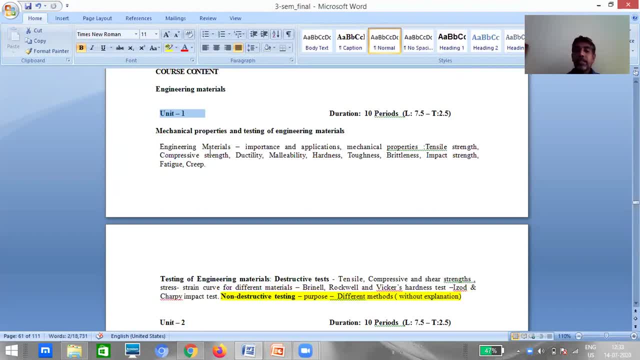 strength, ductility, malleability, hardness, toughness, brittleness, impact, strength, fatigue, creep. all this comes under mechanical properties and we have discussed elaborately all these properties and we are able to define what are these properties are and we are able to list out as well as we are able. 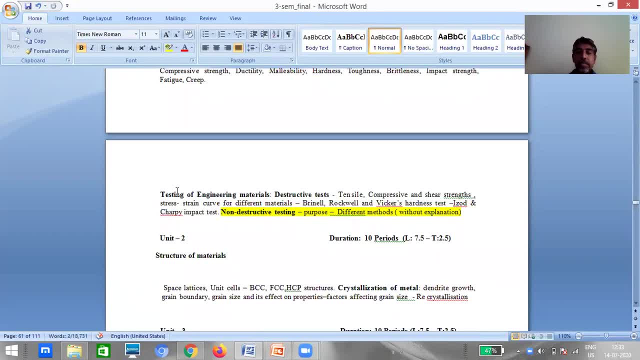 to define different types ofductility during our testing. during our testing and this X T austen Georg students themselves and we later have passed under the 407 criteria that was discussed before. so here are some minutes under design. so weishman dedicated in types ofductility and we talked about rapiddelay test strive. 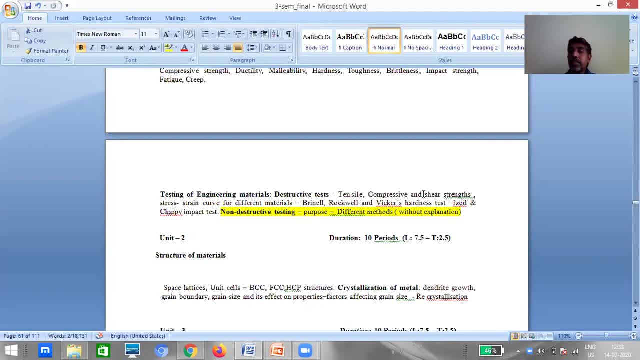 discussed tensile test procedure, compressive test procedure, shear test procedure and later we have discussed the salient features of stress strain diagram for a ductile material and a brittle material, and what are the points that are present on the stress strain diagram and what is? 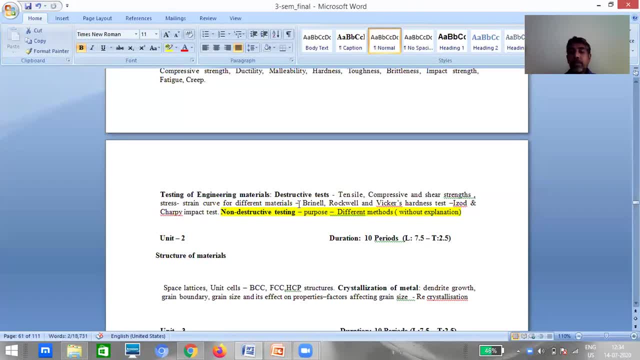 its importance. we have discussed, And later we have discussed, the hardness of the material and how to find out the hardness of a material by using different testing methods. Here, if you see, in the hardness testing methods we are having different types of hardness testing methods that 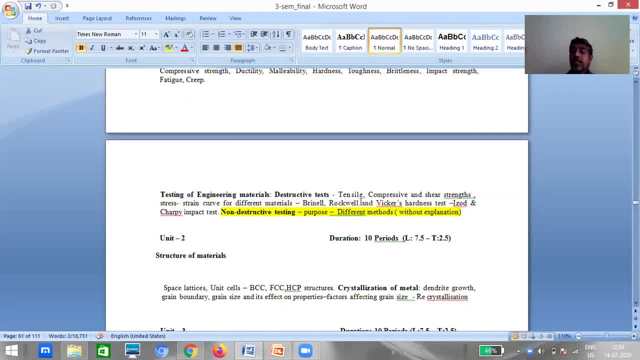 is Brinell hardness test, Vickers hardness test, Rockwell hardness test In the Rockwell hardness test. in the Brinell hardness test. if you see the Rockwell hardness test in this Rockwell hardness test, we are having two types of scales: B scale and C scale, and so what is the difference? 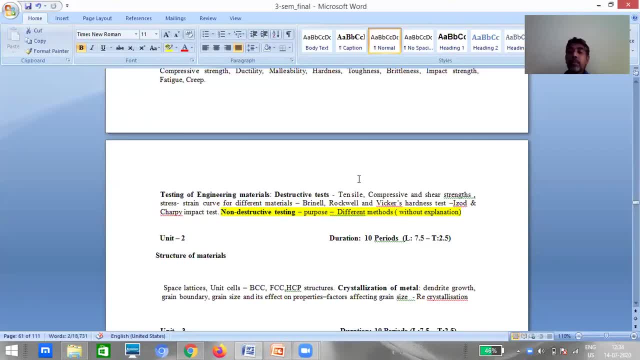 between B scale and C scale. that means how the procedure may change when you use B scale and how the procedure may change when you use C scale. those things we have discussed, And also we have discussed how to find out the impact strength of the material and what are the different types of.